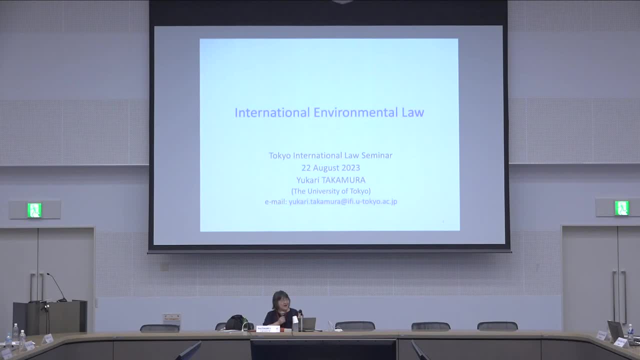 Good morning everybody. Yes, so you were speaking, you know, about the climate change negotiations and there was a discussion in the private sector about the climate change negotiation. There was the participation as part of the international climateных negotiation on the environment. I I may I ask you if you had? 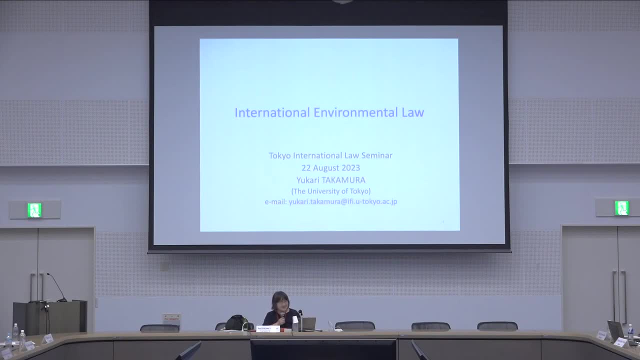 the chance experienced. the, you know, participated in the international negotiation on the environment, For instance, climate change negotiation, or now the plastic convention negotiation is underway. If you had a chance- or currently you are got involved in the negotiation- could you would? you? 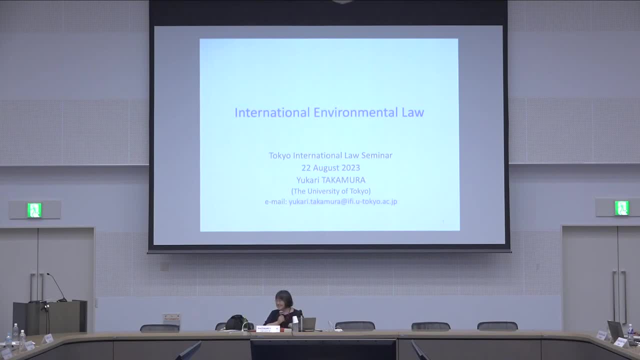 do you have a comment? Sure, Okay, thank you. Okay, thank you. All right, Thank you, Have a nice evening. Thank you, Have a nice evening. Have a nice evening. I ask you to raise a hand. No, 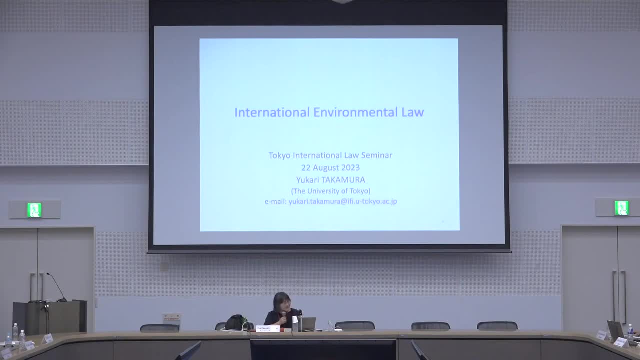 OK, But maybe I think that it is. how can I say my lecture? I wish to start with some kind of quite a brief introduction of the history and the framework of the international environmental law, But the latter part I focus on the climate change negotiation. 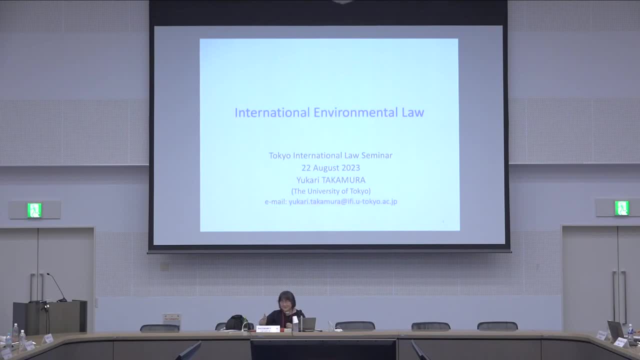 because I think, maybe in the near future or somehow, that you had a chance to get involved in it's quite a big negotiation And also each country has each interest in this kind of negotiation. So here maybe I could start. If you have any question, please stop me whenever you wish. 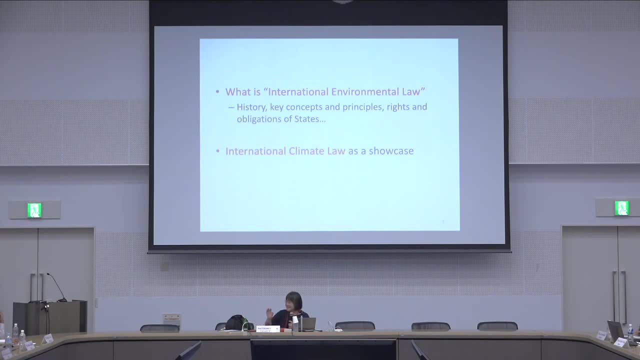 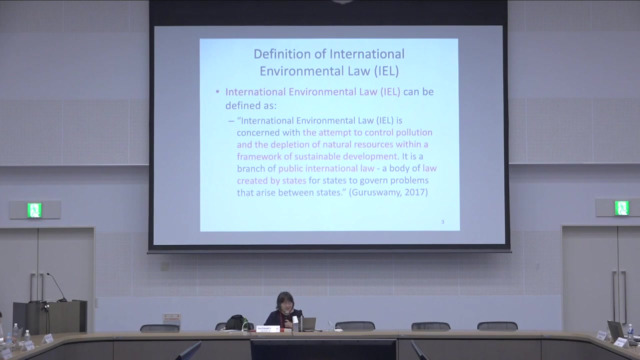 I think it's a lot of time, But I try to interactively. So I think our staff of the Ministry of Foreign Affairs maybe make someone running to give you microphones. So first part is the brief introduction of the international environmental law. What is international environmental law? 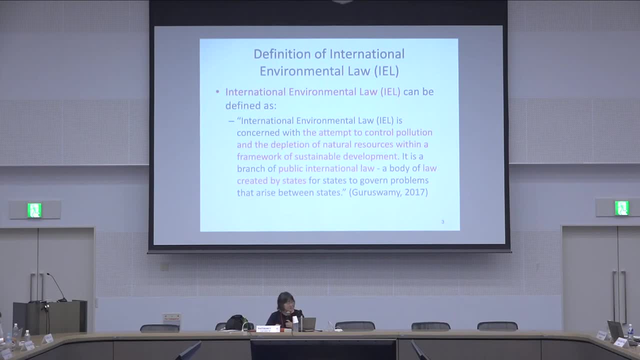 It is defined. it's one way to define that It is somehow the attempt to control pollution, depletion of natural resources, with the framework of sustainable development to address these issue. It is a kind of a branch of public international law to address these issues. 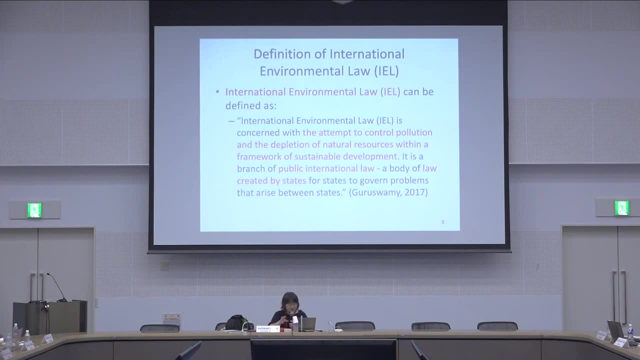 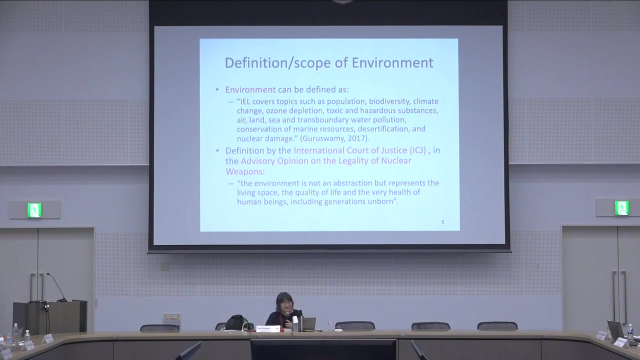 Of course, as you know, the international law is a rule law created by state for state to govern these problems. So it is not a single law, It is a kind of a separate and separate program. But what is now the environment? 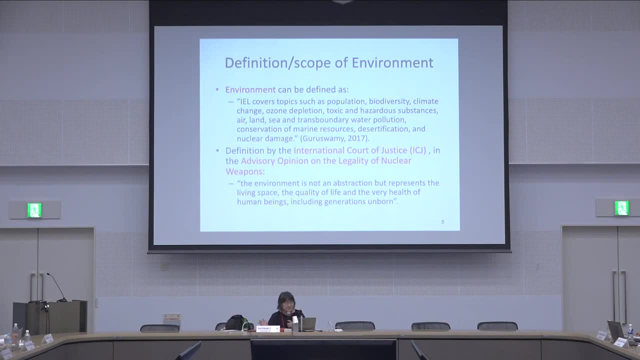 It's quite a broad. Actually, everything is surrounding us, starting with the biodiversity and climate change, ozone depletion issues and chemical and hazardous substances, of course, air, land, sea and transponder. Everything surrounding us, and also the something related to the element of the ecosystem, is covered by this term environment. 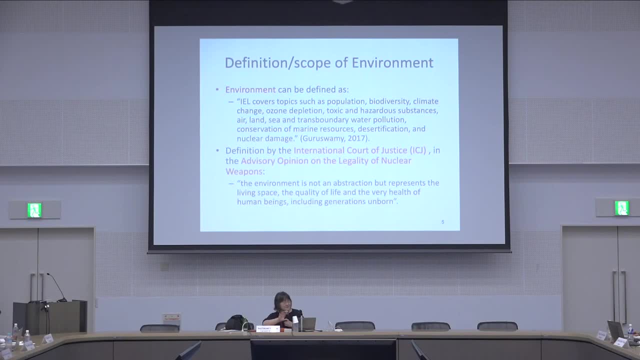 Actually, under the international law- I mean the agreement among the states- the environment is defined quite broadly. I pick up one advisory opinion, as you know that, on legally of nuclear weapons in 1997, International Court of Justice say that the environment is not an abstraction but represents the living space. 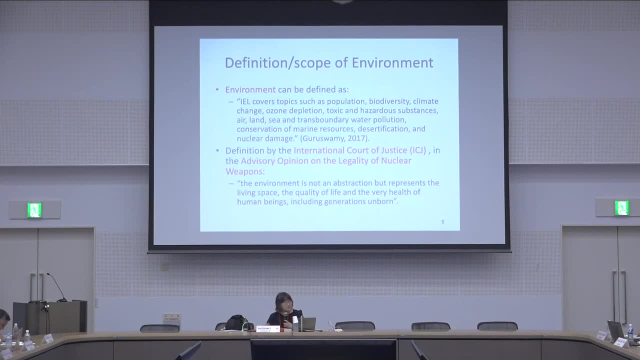 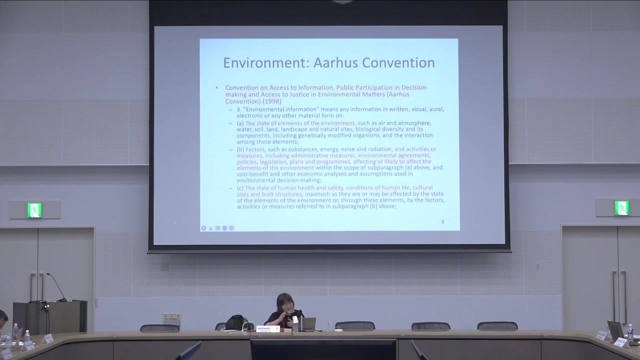 the quality of life and the very health of human beings, including- it is important- generation and born Not only the present generation but also the generation to come. So they Little bit more in detail of what is environment. Of course it depends on the 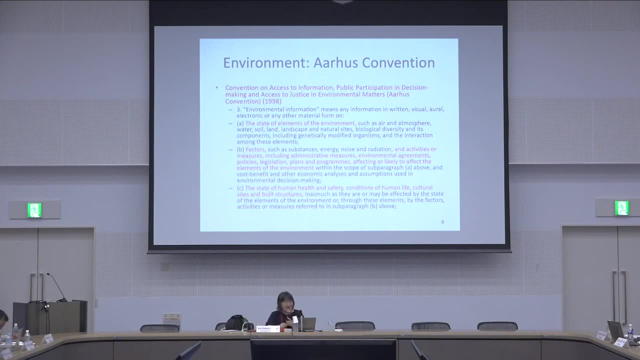 for instance the international agreement, how to define the environment. I pick up here the one of the European Convention. but the European Convention is not a little bit. It's a little bit misleading because it is open to all countries Other than European countries. it is an office convention. 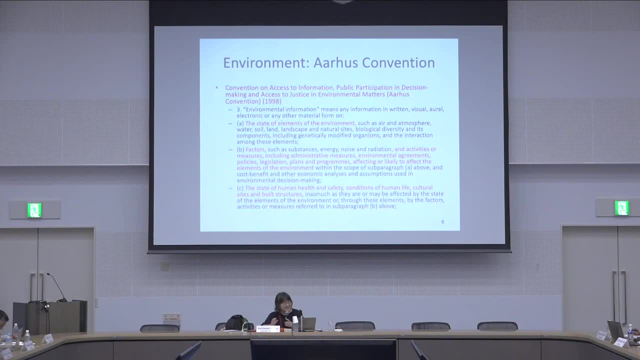 Maybe some of you might have heard the name. It is a convention to ensure the access to information and public participation in decision-making and access to justice in environmental matters. Office is you know, as you know, the name of a city in Denmark. 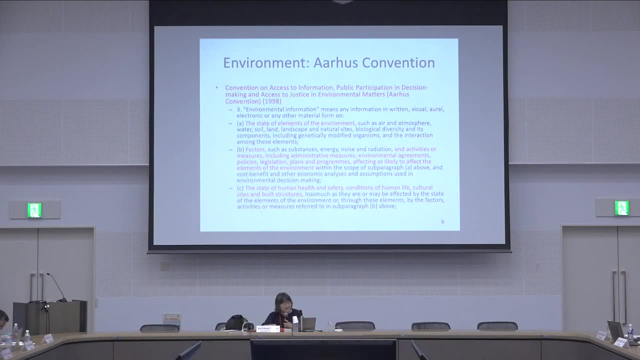 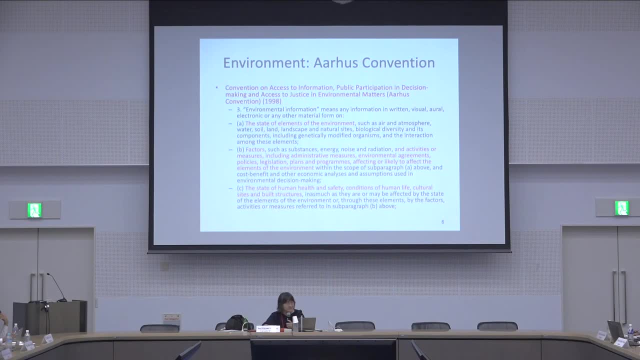 but also the environmental convention. here I mean this convention also covers not only the element of ecosystem or constituent of the ecosystem, but also the element of ecosystem or constituent of the ecosystem system, but also the something to impact the, the quality of environment, for instance energy use. 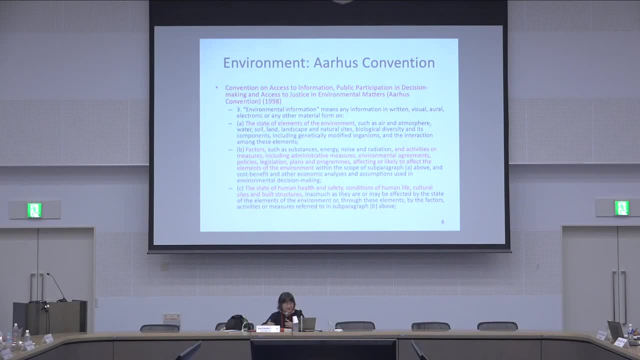 noise and any activity to have a potential impact on the element of the environment. so you can imagine that it's quite broad as a scope and also not only pure environment but also the, as you know, that the house may be impacted by the degradation of the environment. 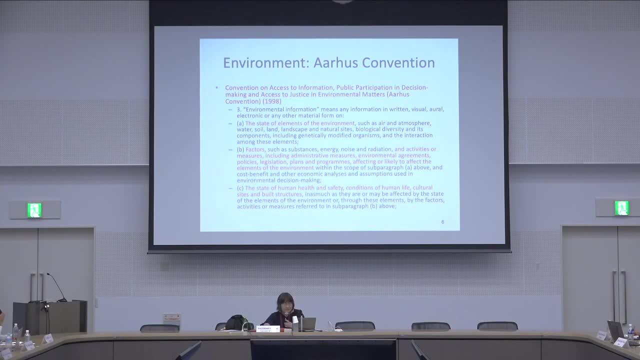 so the health and the safety and the condition of human life and the cultural site and even built structure is considered as a you know, the scope of the environmental information. so i, i, i, if you, just i could say that under international law in general, i think the environment 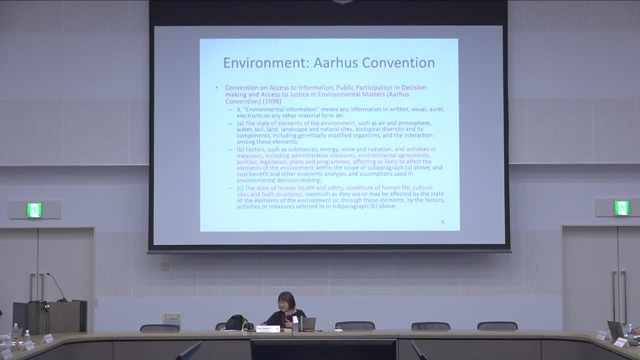 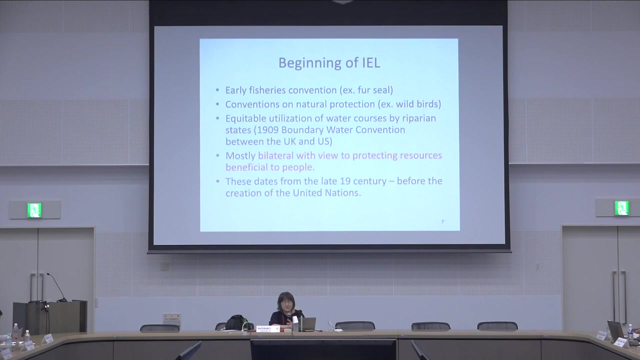 is broadly defined, of course, finally, according to the each international treaty or convention to define it. so now the how this international environmental law developed or evolved over time. so it's is a not so old area of the international environmental international law, if i may. it started the fishery convention. i understand that today you had a class you had. 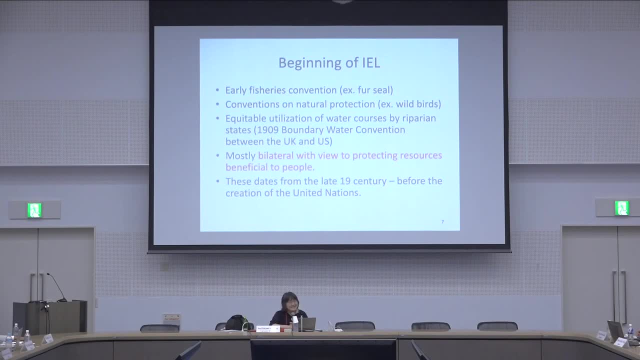 that speech on the law of the sea. so the a part of law of the sea considered, uh, you know, a part of or international environmental law, because fishery convention one objective would conserve the fishery sources. so here the. i see the one example, the, among the united states, in russia and japan we had the first sale: conservation conservation. 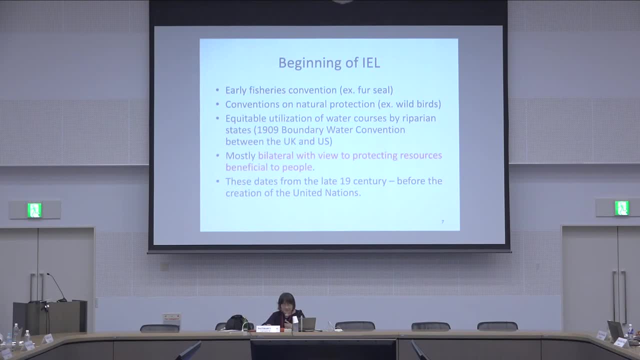 fossil in the end of 19 centuries. so another example is as conservation of the natural nature or conservation the species, especially early time of the international environmental law, have a objective to protect the species and was the or variable for human uses, for instance here the i pick up one convention. 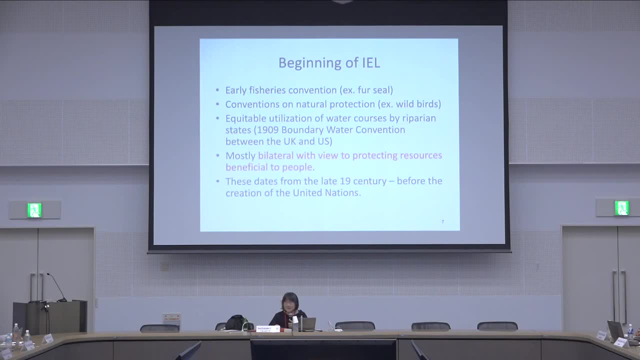 as the example is that the, i think between the belgian and a couple of european countries concluded the, the convention to protect all, because all you know actually eat the insect to have. you know the cause, the damage to the agriculture. so this, uh, this first sale convention, and also all. 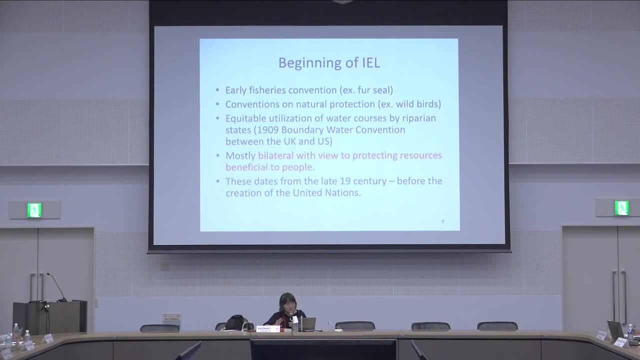 as, uh, you know, variable and the species for human activities. so the first, um, how to say, motivation of international environmental law is that how to protect the nature and species which has a value for human being. almost at the same period to the館, we have some kind of, you know, the international pollution issue, especially between two or a couple. 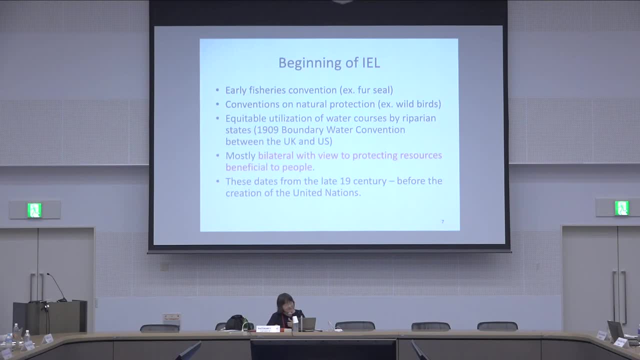 of countries here, the i pick up one example is that the uk and the us. you wonder what is the water boundary between uk and the us? it's atlantic now it's. it's a kind of a treaty, the water convention between the canada and the united states at that time. so you know the. 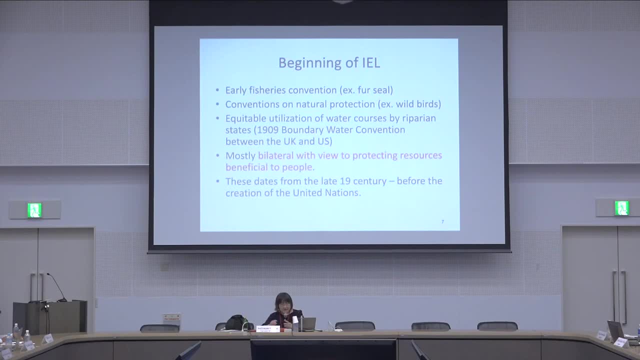 interwar international water is very important and so that to conserve the quality of water and the volume of water, that is the objective of this convention. so, as i said that at our timing of international law, international environmental law, the main purpose is that to protect the valuable resource for human being and also the usually or generally. 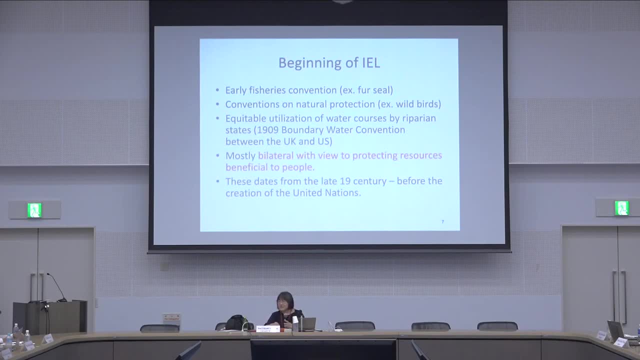 speaking that the scope, geographical scope, is quite small and uh, bilateral, or the at least at most regional. so still the we can see some kind of trace of the international environmental law, even the the uh the end of 19th century or the beginning of 20th century. maybe the first case that the international tribunal made a judgment is the 12th matter case, that is, the case uh, a dispute between the united states and canada. that is the one of the uh refinery uh emitted sulfur oxide and which go to or go beyond the the boundary uh to the united 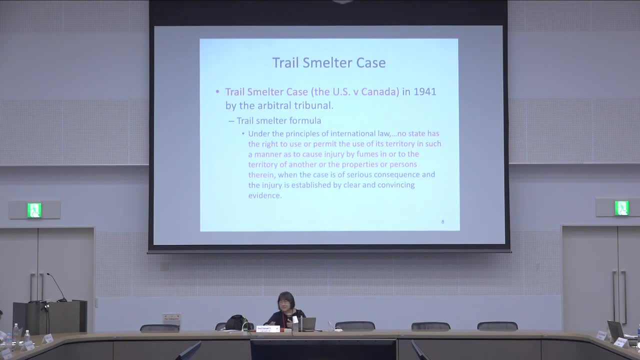 states. so that's cold, the, the damage to the agriculture, production, the forest. so the united states wish to get the compensation or they stop the operation of that refinery. so the, the two canada, actually, they accept that the this refinery cause damage to the united states. but the discussion or the dispute point is: 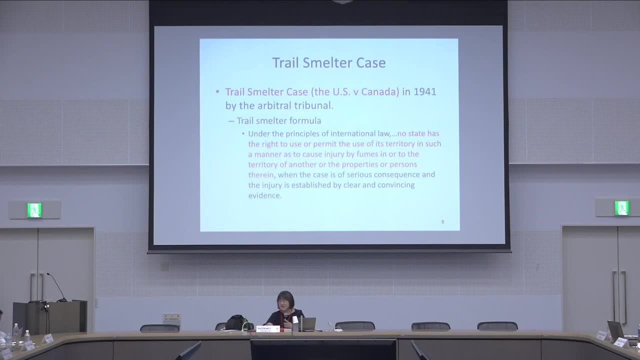 that the how to define the amount of compensation, or the your heart is Studios. and there's this arbiter tribunal deliver a judgment in 1941.. this is uh often called the traveler case and the- it is a typical formula- which have a quite a significant impact on the development, future development, of international environmental law. here's. 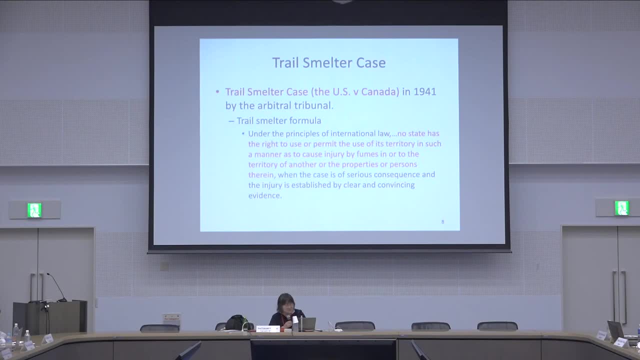 the term that Maserati hugh qualified the first general household value sign, Aucklandائy of international fundamental law. here's uh income in the population over the next 12 years. hugh wanted to be shut away already, thank you. Here you can see that no state has a right to use or permit the use of its territory. 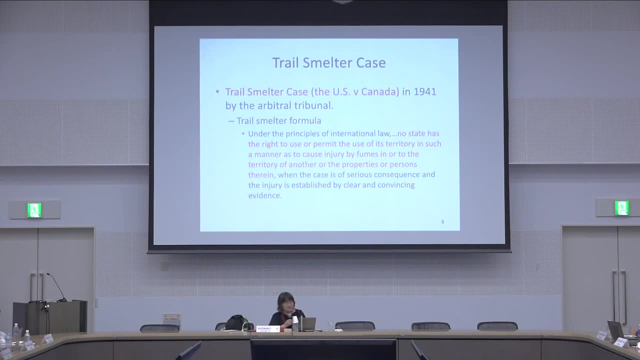 in such a manner as to cause injury by fumes in or to the territory of another of the property or person therein. That means it's a kind of a denial of the absolute sovereignty. Absolute sovereignty as you know that the sovereign states are full and absolute power. 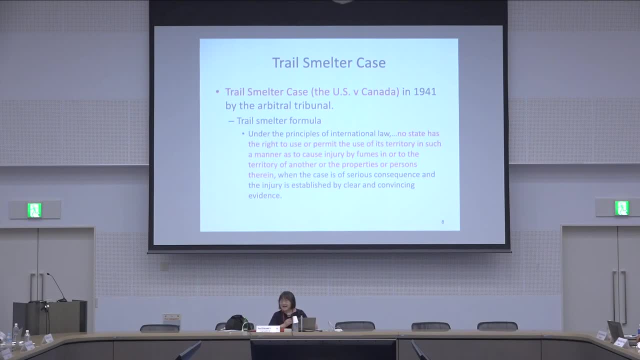 to control everything in its territory. Actually, in the context of air pollution here it is a first case The tribunal deny that there is no absolute sovereignty. It is some kind of imitation If the activity code kind of damage to the another country or the environment to in another country or 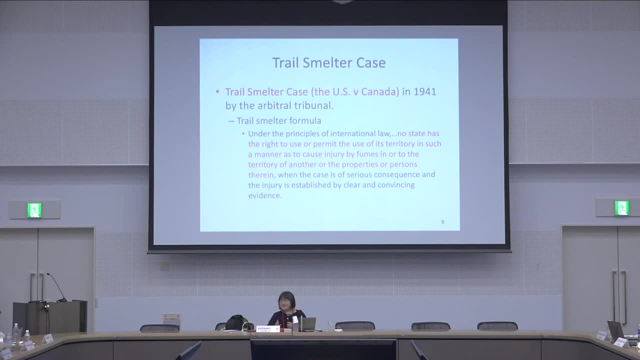 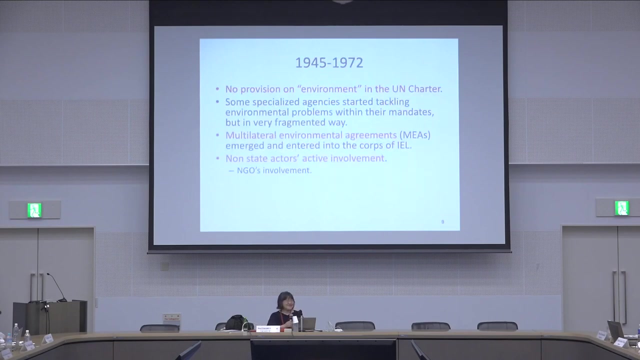 here the property or person, in that case the X- there is limitation of the exercise of the sovereignty. so it is- this formula is very important that you can see later, because now it's become its origin of the, the general obligation of the state under the international environmental law. so maybe we come to 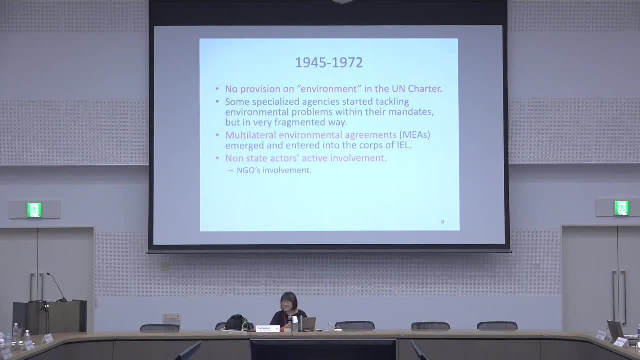 more recent here, the 1945. it is, as you know, that's the end of World Second War and also the the year of the establishment of United Nations. I think that the you know, you, you have a chance to see the United Nation Charter you. unfortunately, today we did no word: environment, no chapter and no clothes of. 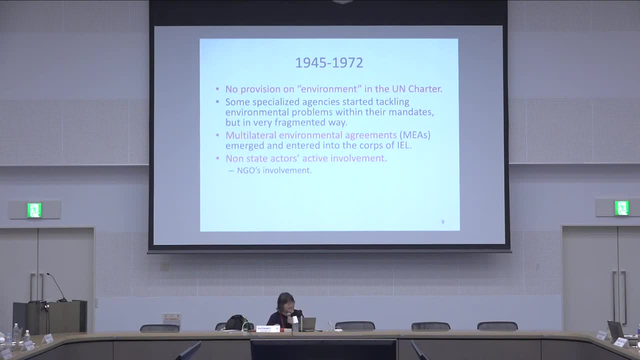 course we have a you know word, human rights and but no word environment that show that, some kind of perception of the state at that time that how the most important or urgent issue that state face. but but from the 1950s some specialized agency, especially here I like to cite the one specialized. 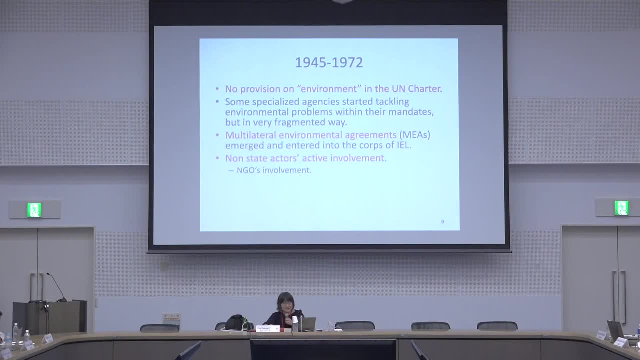 agency, as international maritime organization IMO started tackle the environmental problem, especially the marine pollution from the, you know the oil spill from tanker or ships. so they try to elaborate international agreement. so but such kind of you know, trial or the undertaking that happen but it's depending on the each. 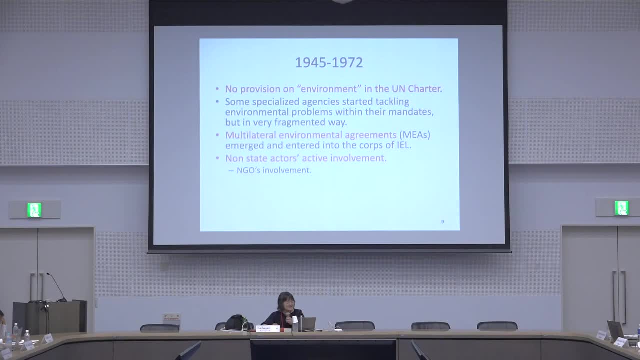 international organization. so it's really not a systemic way and rather the fragmented way but that still they this over towards. in 1960s and 70s a couple of international environmental agreement has, in order to cause a change in the international environment, area of international environmental agreement has emerged, especially in the late 1960. 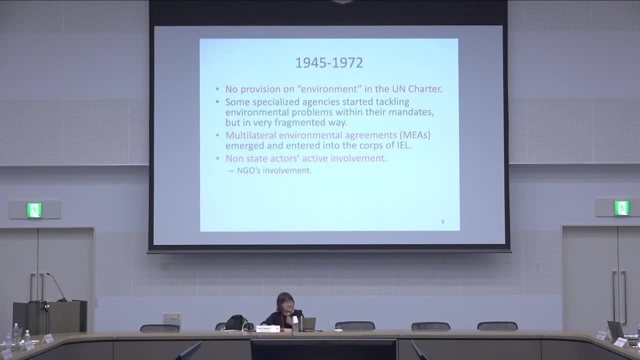 and at the beginning of 1970 we see a very fast generation of nature protection, as you might know, that Ramsar convention to protect the international wetland of the international importance, and also the CITES convention on the, you know, the regulation regulating the trade in endangered species, that is you. 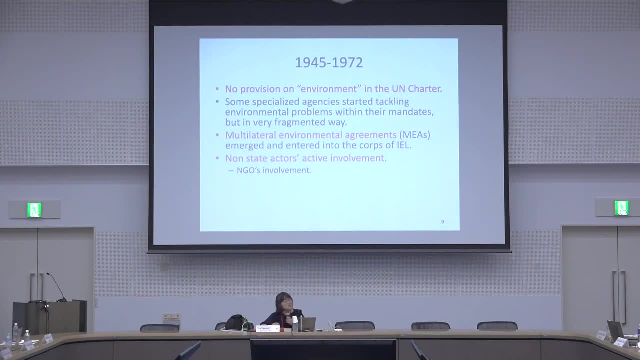 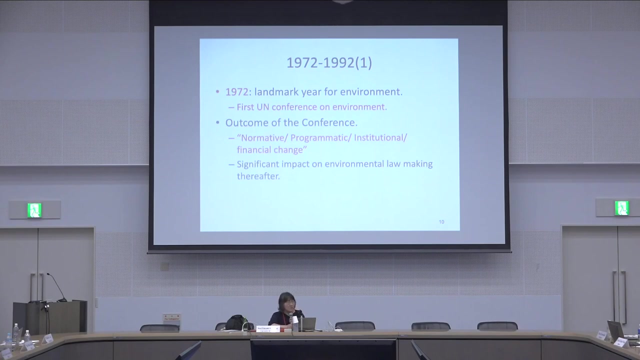 know quite early. you know, in terms of environmental or modern environmental treaties, I could say that's the more. maybe the one of the most important year is 1972 for the development of 1972. they held the first United Nations conference specifically addressing the environmental protection at the time. as you know, that's the especially developed. 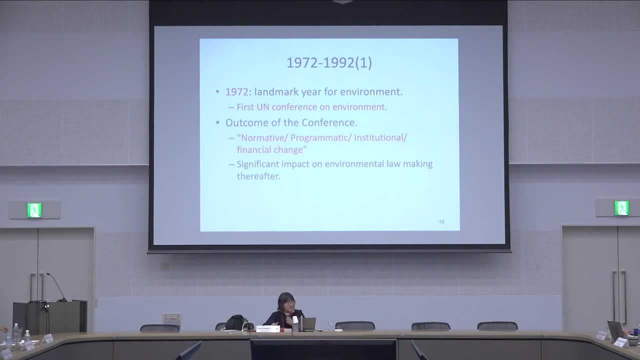 country faced the public nuisance issues. you might know that the mercury pollution here in Japan and others. so this air pollution, regional air pollution and some kind of acid rain phenomena in Europe. so the, the this 1972 you any confluence on human environment? for for the first time address the specifically the environmental protection, but still 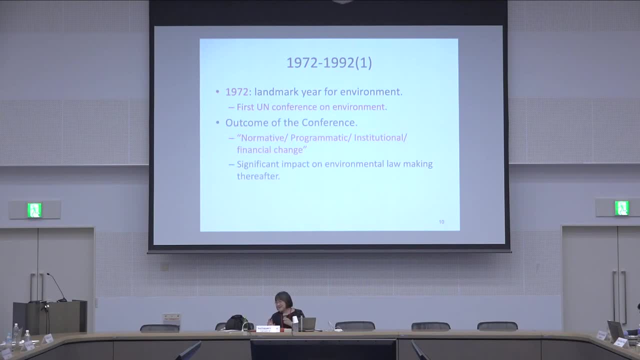 there is some kind of gap of perception because they developed a country somehow, you know, promote more regulation for the environmental protection, but at that time still the developing country facing the you know, the underdeveloped, and situation in the lack of the, the you know development, so the, the you know, there is a kind of gap. 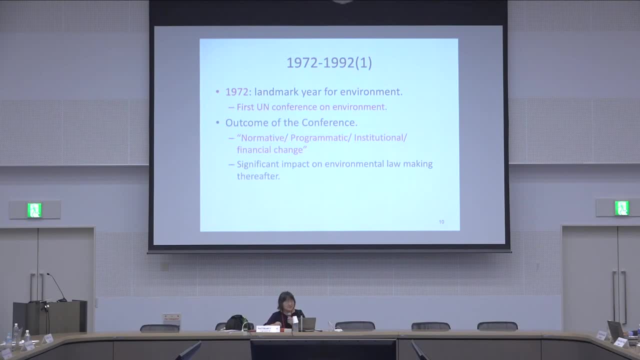 between developed and developing countries on how much important on the environmental protection. but still this year is at this conference is quite important because there are some outcome here. I've cited four of the outcomes in this conference, since I don't have time right now for the participants, so this is the end of the 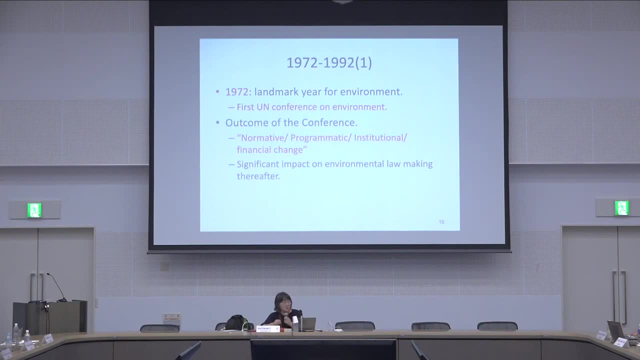 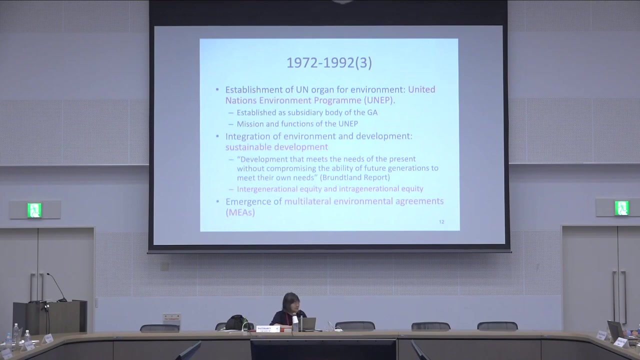 is that they elaborated the somehow the two doesn't principle to frame the international environmental law. I pick up in some example later. and the second important outcome is that I think you should know the name is that the United, based on the agreement made in this 1972 United Nations Human Environment Conference. 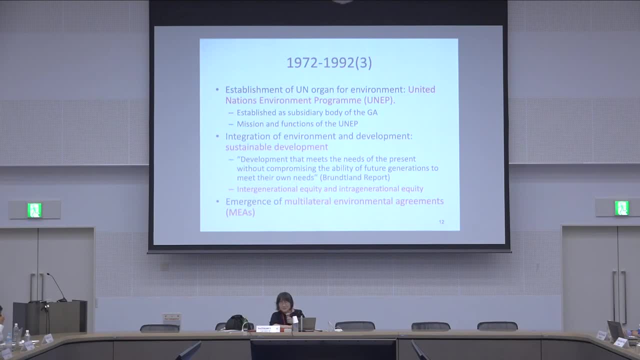 So UNEP has a very active role to promote the finding of new environmental issues and somehow coordinate activities, especially within the framework of the United Nations, relating to the environment. Also- this is kind of you know- the assisting organization, together with the UNDP. 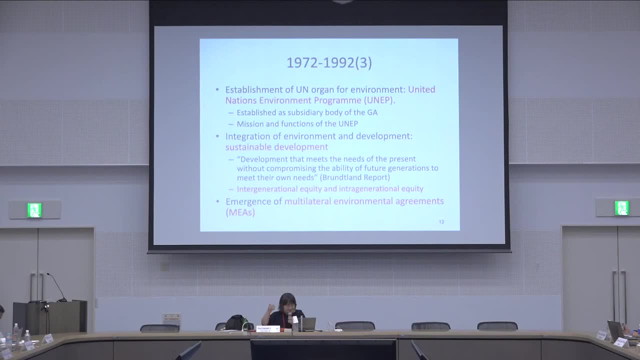 When the developing country wish to somehow apply some kind of funding, for instance with, you know, global environmental facility and others, and that the UNEP assists the developing country in the elaborating the document and, you know, enhancing the activity. 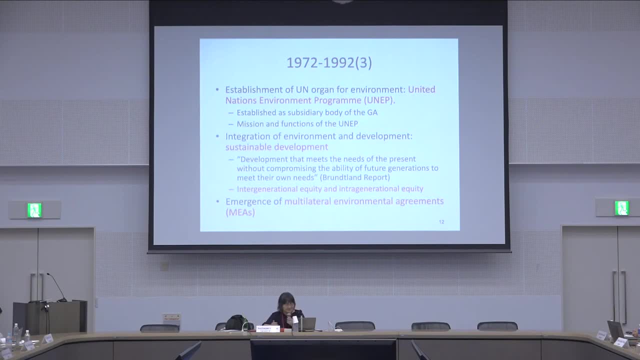 which is the UNDP, With the project adopted. So also this UNEP supports the international negotiation, especially on the new environmental problem. For instance- I think I'm going to speak a little bit- but the Convention on Biological Diversity, it was adopted in 1992.. 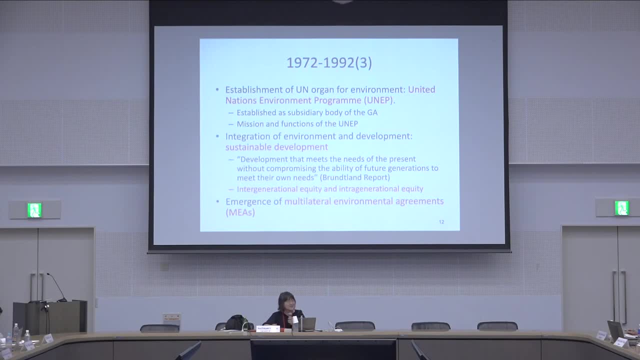 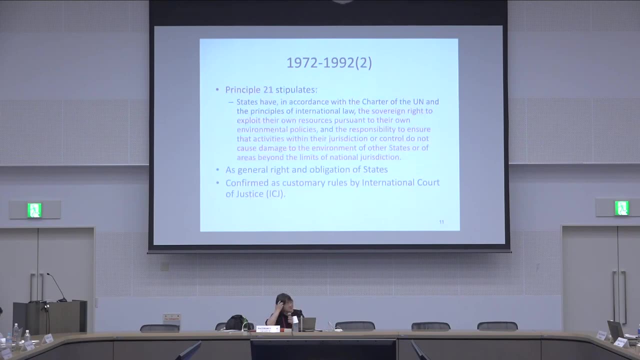 That was negotiated, supported by the UNEP Secretariat. So I just a little bit back to the 1972, because one of the first important outcome is a normative outcome. I say that it's elaborated. the conference elaborated a series of political principle. 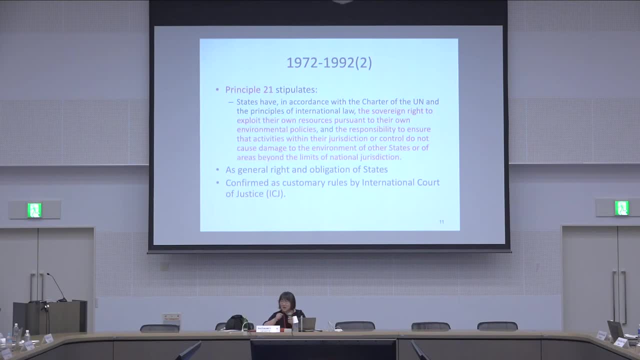 but the important from the sense, from the perspective of international environmental law, is because it's it's getting legally binding-ness over time. So you can see some kind of similarity between the 12th model formula here, but a little bit modernized way. 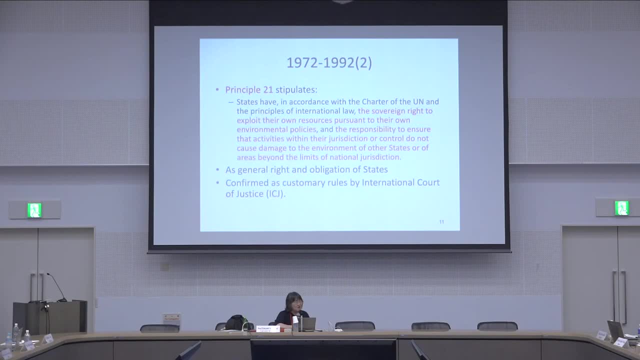 Here the principle 21 of the Stockholm Declaration. I say this: 1972 UN Conference on Human Environment is held, actually the Stockholm Sweden, so that the name of declaration is often called the Stockholm Declaration. This declaration contained the two thousand principle. 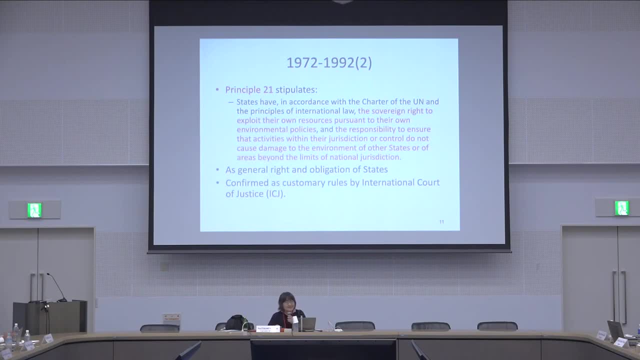 One of the principle is here the accept or recognize the sovereign right to exploit their own resources, At the same time the responsibility to ensure the activity within their jurisdiction or control do not cause damage to environment of other state or the areas beyond the limit of national jurisdiction. 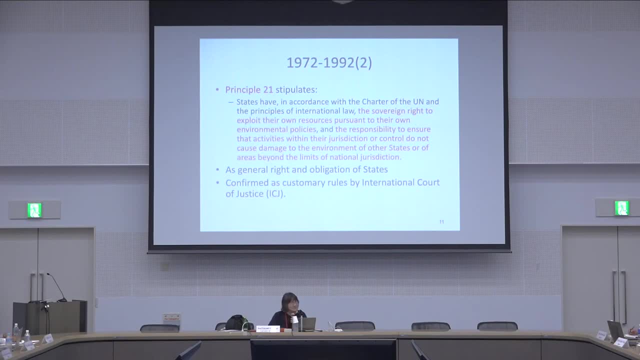 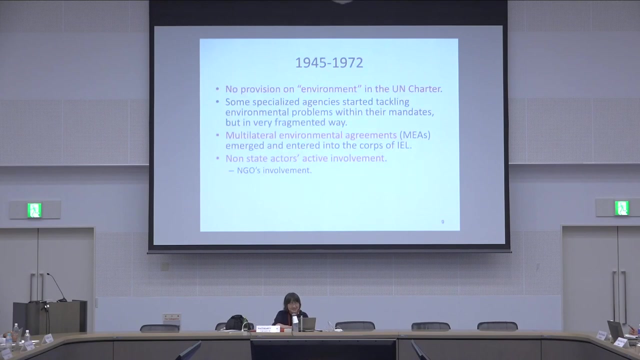 It's really, you know, the some kind of development from the 12th model, because the latter part, the part, refer to the responsibility. Here they talk about the. you can remember the 12th model case, The activity within the country. 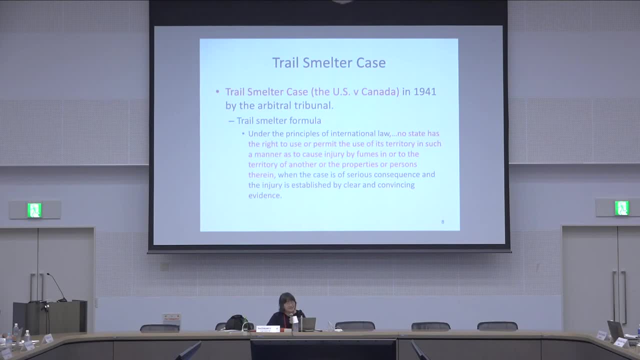 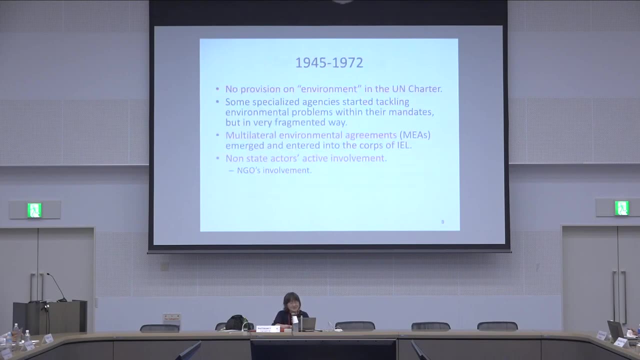 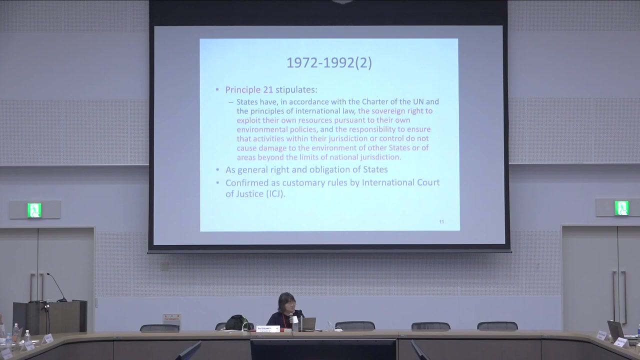 not, do not cause any injury here in the context of air pollution, but not injury to other countries. Quite a similar way, but a little bit modernized way Here: the activity within their jurisdiction, or control jurisdiction. you mean that, of course. 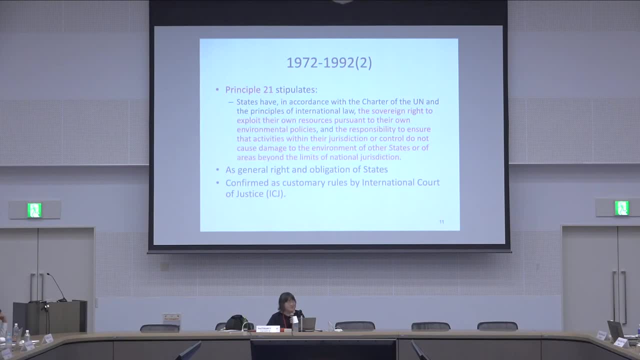 the, you know the territory, of course include the territory, but here jurisdiction mean that they cover the, not only territory but also the executive. you know the exclusive- I'm sorry, exclusive- economic zone. activity within the jurisdiction countries do not cause damage to the environment of others. 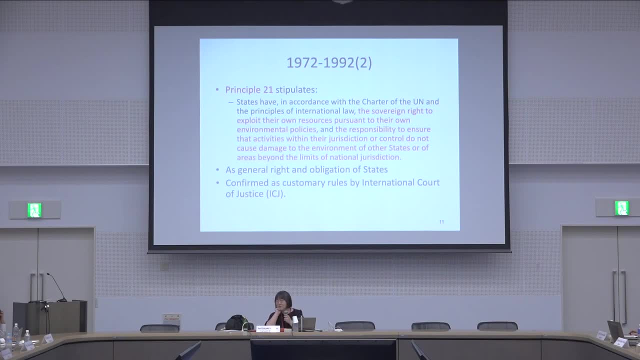 Also, I like to say that there is a word of control. What is control, You know? for example? I think that there is a word of control, for example, a bird, for example in the question. we do not have a bird to leave their territory. 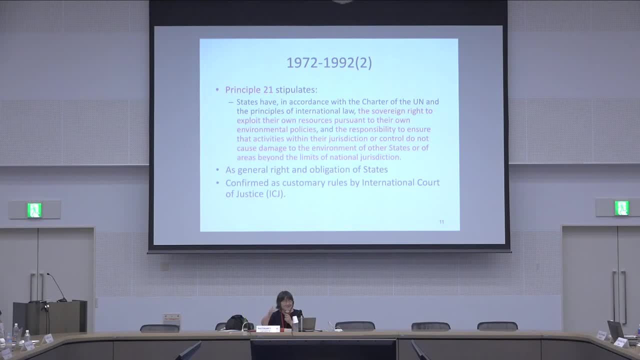 we have a bird to stay, but there are birds that you know. the birds are not living in the territory of others, Right? So I think that's the whole point. So individual as well. You are out of your countries, but still somehow you are. 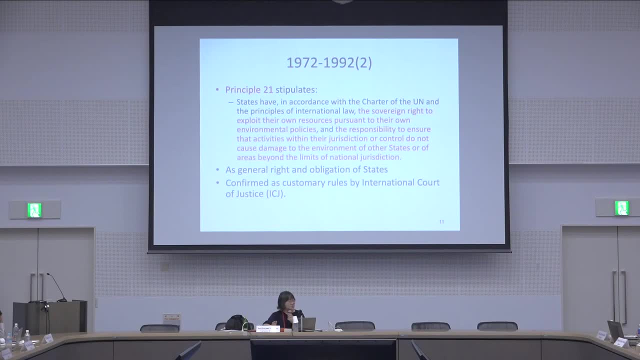 still under the jurisdiction of your countries. So here, for instance, you can imagine that the ship outside of the jurisdiction of the registered country still, even outside the registered country, have to exercise to ensure that these ships, registered ships, not to cause damage to marine environment. 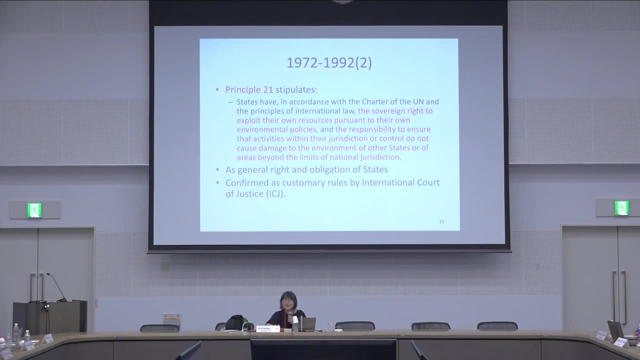 So then you can see that the coverage of responsibilities, scope of responsibility of state not to cause damage to the environment of other country and outside of the national jurisdiction, is actually the extended and expanded, not only the activity within the territory And also another point of expansion- yes, I already. 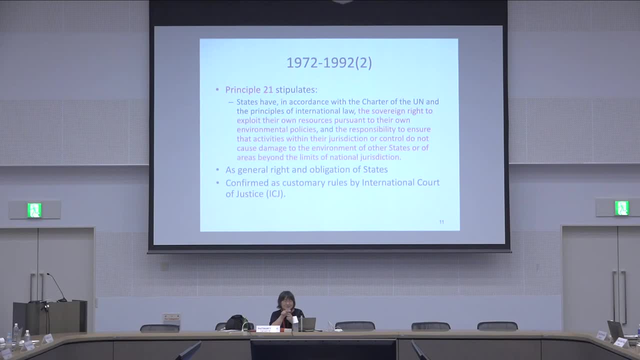 mentioned that in the end of this principle, not only you know environment of other country, but also the area beyond the national jurisdiction. I think I understand that Nishimoto sensei- Professor Nishimoto, you know- introduced you that BB and J you know. 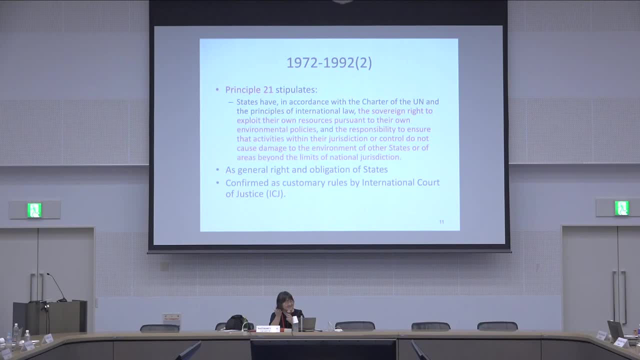 the. you can then understand that it's a high sea area. it's out of the, beyond the limit of national jurisdiction. So then, but as ships- you know the navigate over high sea- yeah, you know the registered country- have a responsibility. 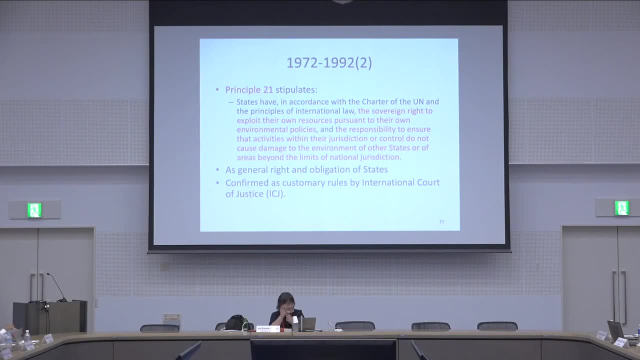 not to that, you know, the this registered ship cause damage to the high sea environment. So this is quite important because, As I already mentioned, it is already confirmed by the International Court of Justice and the advisory opinion of the legality of nuclear use. 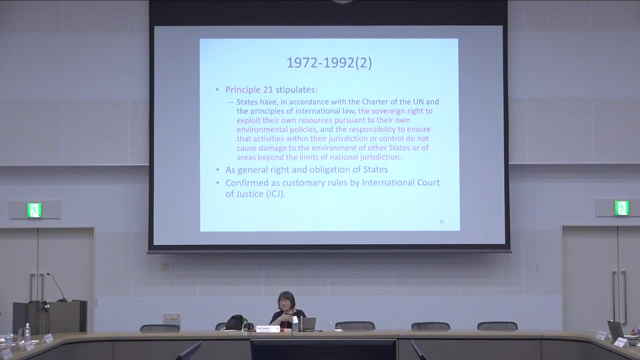 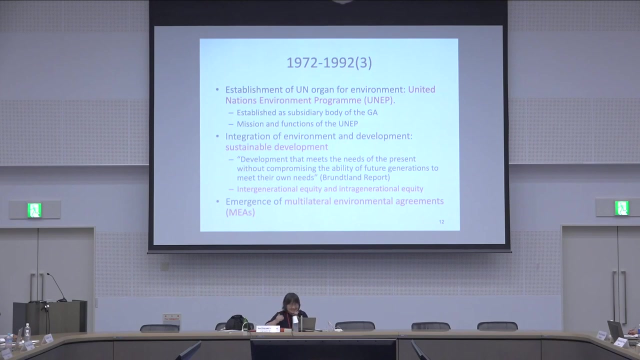 it has already become a customary law which applies to all countries, even though there is no specific international convention. So I think I have to rush, but I'm almost finished. but we have a very important concept in the 1980s. 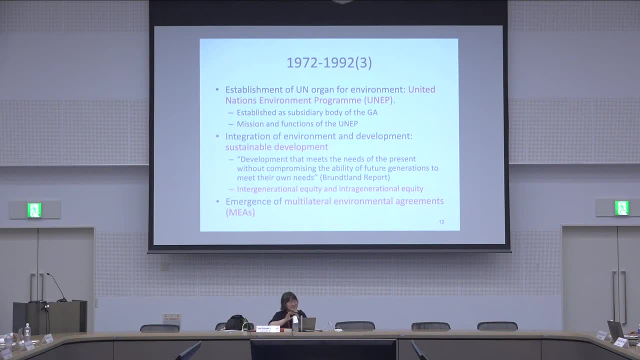 which is the sustainable development. Of course, as you know, SDGs are political goals for all countries toward 2030. But here, in terms of In legal terms, the concept of sustainable development is quite important. I think we see later in the context of integration principle. 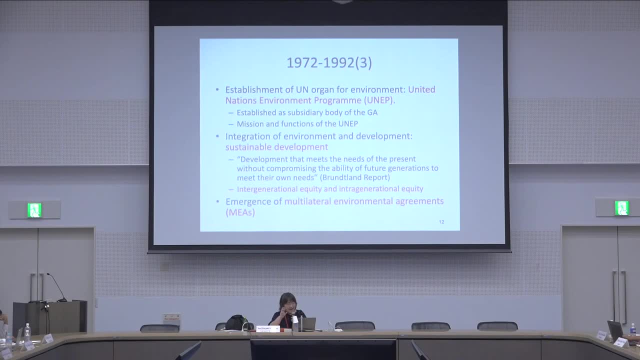 But here I'd like to say that in the 1980s we have an emergence of the sustainable development concept on the one side, and it's a political goal, but on the other side it's something with the concept, with legal implications. 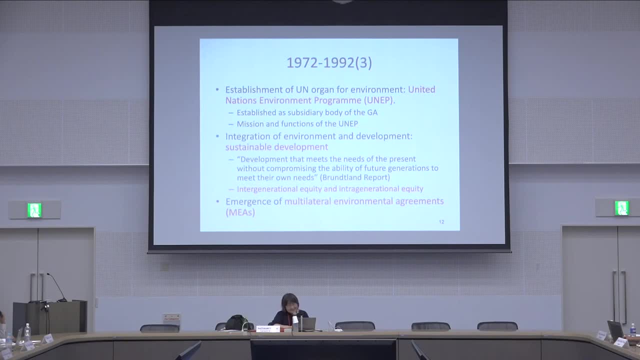 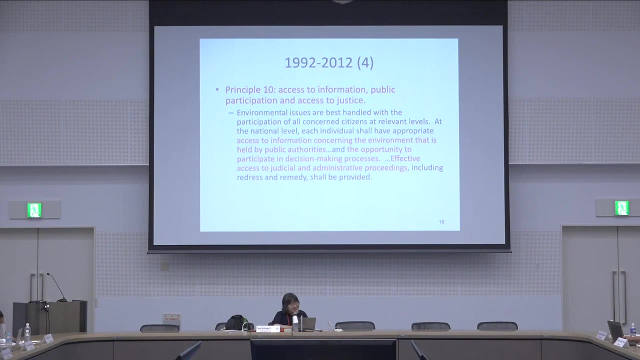 And since 1980s and 1990s we have a lot of machado environmental agreement. I just have put some list, I think from the slide 20.. It's plenty of international agreement. It is only multilateral, of course, if we include the regional. 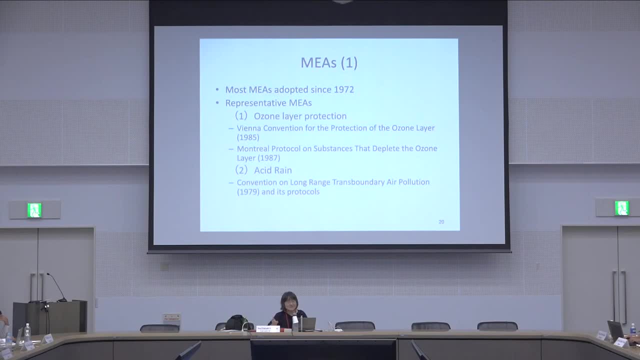 and bilateral, And since 1980s and 1990s we have a lot of machado environmental agreement And since 1990s and 1990s we have a lot of machado environmental agreement. I think it's more than 1,000.. 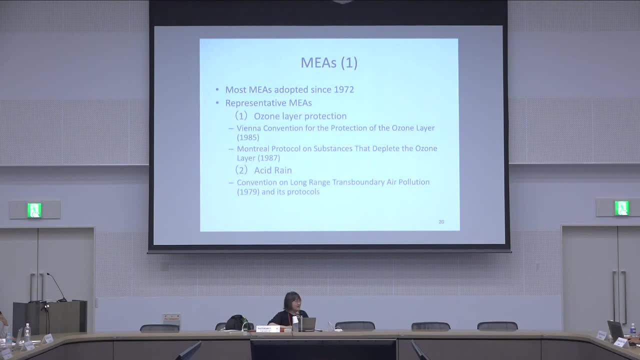 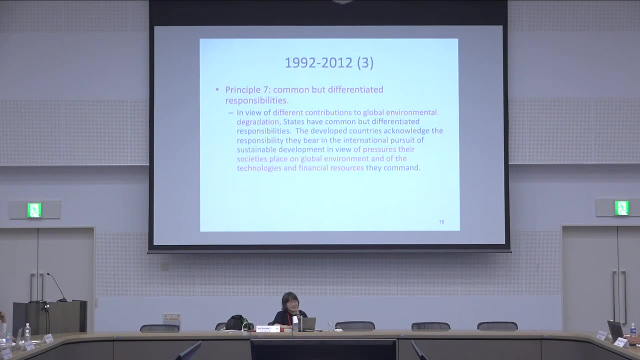 But here I cited the representative multilateral environmental agreement. So, coming back to the 1992, because the second landmark year for environment is the 1992, 20 years after this UN Conference on Human Environment, Maybe you might know that the 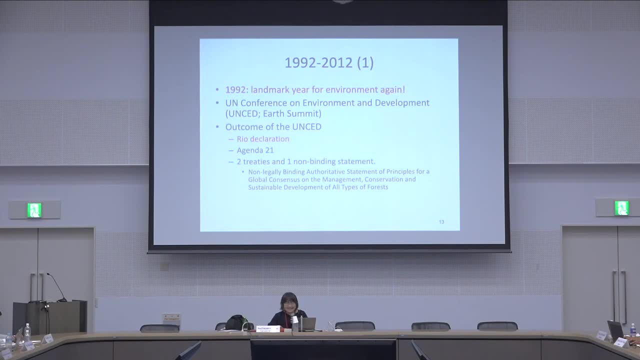 Why is it called the second landmark year? Because it was held in Rio de Janeiro, Brazil, so it's often called the Rio Summit or UNSET UR Summit. It's the first time that the UN deal with the environment together with the development issues. 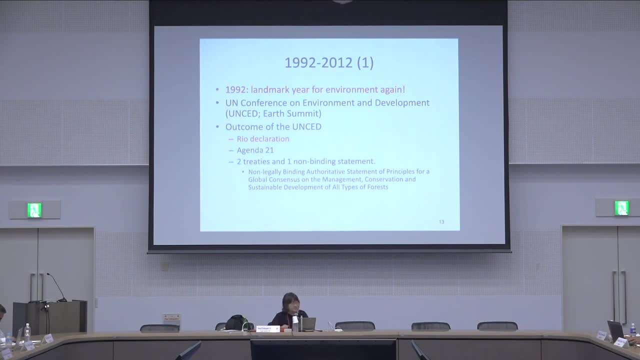 So that deliver three very important outcome. One is normative outcome. in Rio Declaration- That's also the, You know contain the dozens, the 20, around the 20, around the less than 30, but the 2,000 principle. 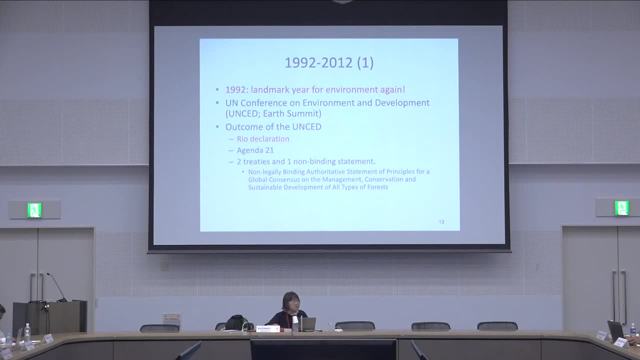 And also Agenda 21 is action plan for all countries. And, as I said at that time, and the two important treaties I think we have now is: one is the Convention of Biological Diversity and another is United Nations Framework Convention on Climate Change- first climate change conventions. 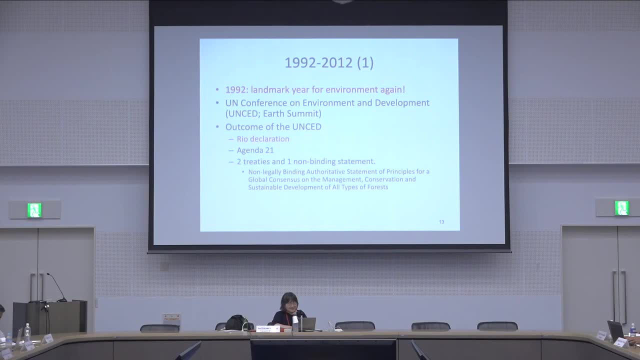 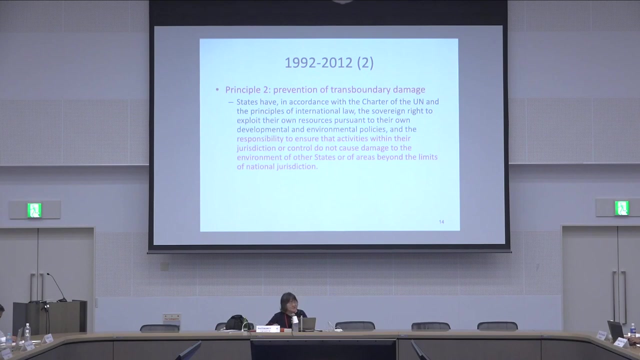 So this real declaration contained, as I said, the quite important pillar principle. It is, of course, this real declaration a declaration non-legally binding, but some have become legally binding. One is already mentioned that quite a similar formulation was the Principle 21 of the 1970,. 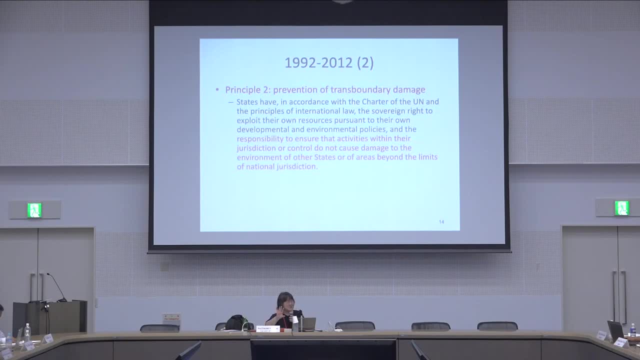 to Stockholm Declaration. If you can compare two texts- I couldn't say now due to the lack of time- but if you look at this Principle 2 of the 1992 declaration and previous one, this Principle 21 of the 1972,. 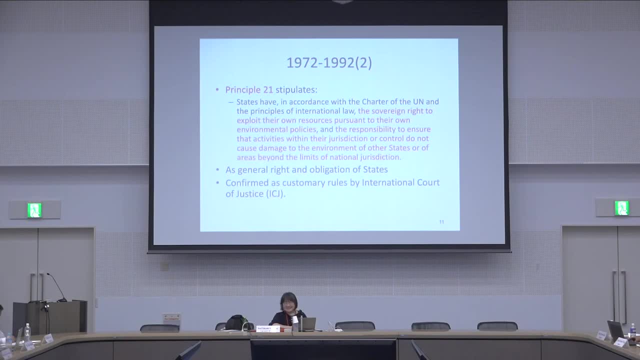 there is only three word difference But you can see what is different. But according You know, the broad sense is quite similar. especially the latter part is the same wording as the wording used in 1972 declaration. As I said, it's already get legally bindiness over time. 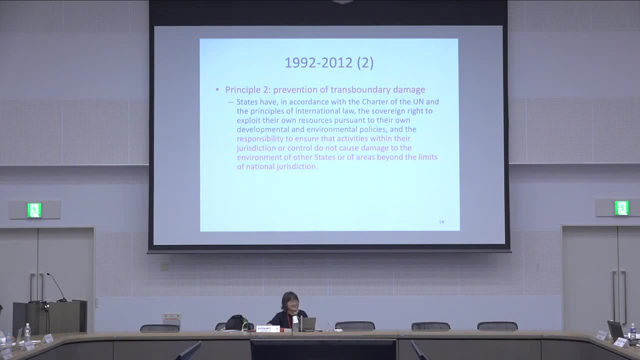 at least until the late 1990s. This real declaration contains, as I say, the basic principle four of the international environmental law. So, as I already told, prevention principle And the second maybe it is quite well known, especially when you do some negotiation. 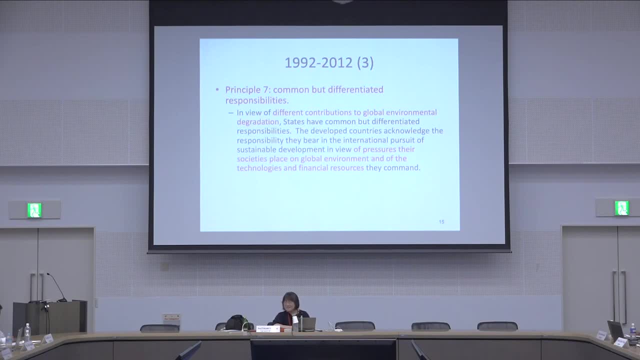 of course, environmental, but also the development, common but differentiated responsibilities. Responsibility is common, common facing and the global environmental issues, But the degree extent of responsibility differ from country to country, especially here, the differentiation between the developed country with the capability. 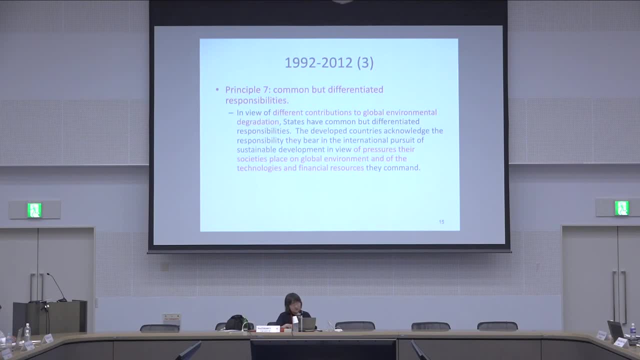 and also responsibility to pollute, to cause a pollution, And a developing country is, on the other hand, So often if you go to the environmental negotiation, this common but differentiated responsibility a key principle, because that is make the negotiation or, how can you say, elaborate the specific right. 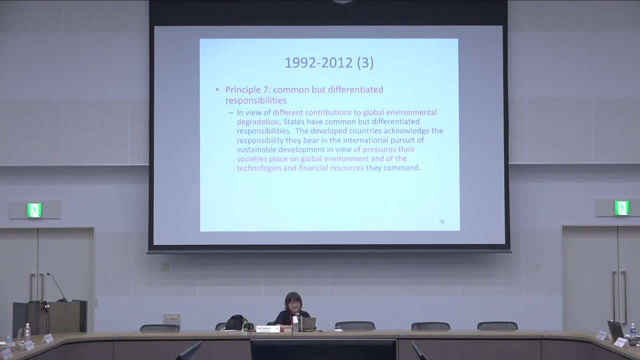 and obligation under the negotiation I think I let you know in the context of climate change later. So the other, the principle 15 of the new declaration, is that is also, I say, quite common in the domestic national law of maybe your country and the precautionary approach. 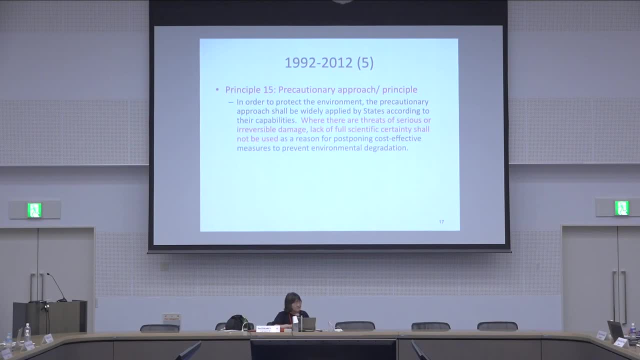 and the precautionary principle. So often the environmental issue involved the scientific uncertainty. no, 100% of scientific certainty, But in such a case if we do not know nothing and sometime later we face quite a serious damage due to such problem. 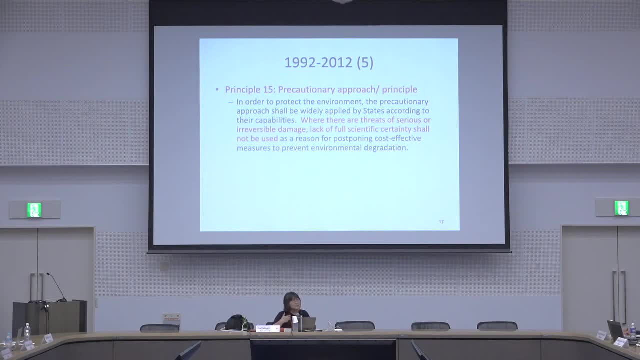 So this is some kind of precaution: require precaution, The country have to pay more attention even though there is no 100% of scientific certainty. So where there's threat of serious universal damage, in that such a case lack of full scientific certainty shall not be used to postpone. 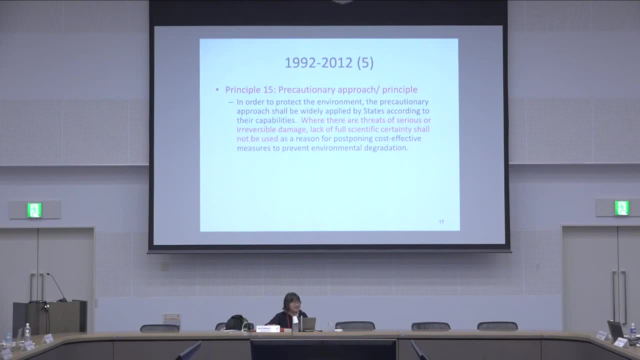 postpone cost effective measure to prevent environmental degradation. I think such kind of issues are quite you face, you know. you should know some, For instance the- I pick up the example in the context of plastic. Of course, the plastic if it is. 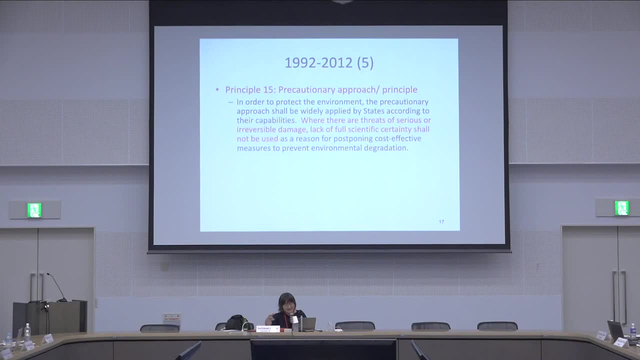 you know this. I can say they emitted in the ocean. that's pollute the ocean. But sometimes the you know, scientists discuss the you know plastic. you know the waste, the over time that you know they create a very micro plastic. 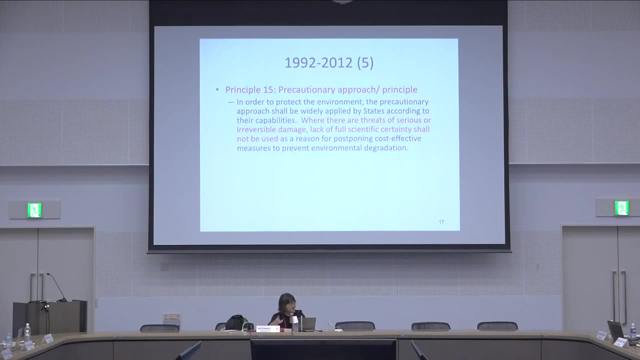 It is, of course, the end of water or in the ocean there's maybe fish eat or the kind of micro plastic, And of course we eat fishes. What is the impact on our health? What is the impact of the ecosystem, including fish? 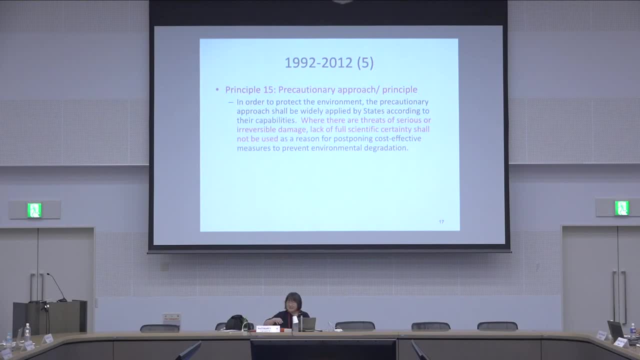 Such kind of thing. still there is a difference of view among the expert. So in such a case we could say that the that you know, the all full scientific certainty, but still we take some, please, some caution, precautious action now, for instance in case of japan and, uh, quite a number of country, uh, you 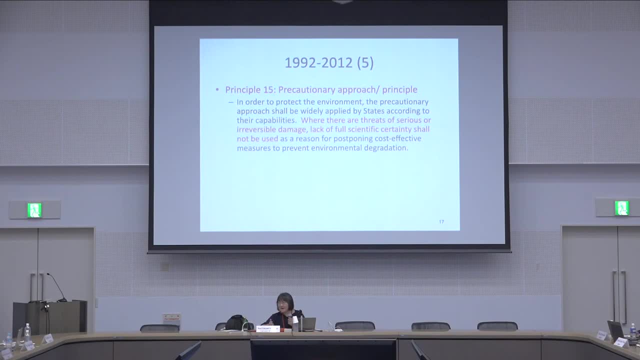 know, prohibit, prohibit the use of microplastic and some kind of washing, you know, product, because that's, uh, you know, directly released to the ocean and the river. so that's the, uh, you know, such kind of precaution i mean, already made even though there is no full scientific certainty. 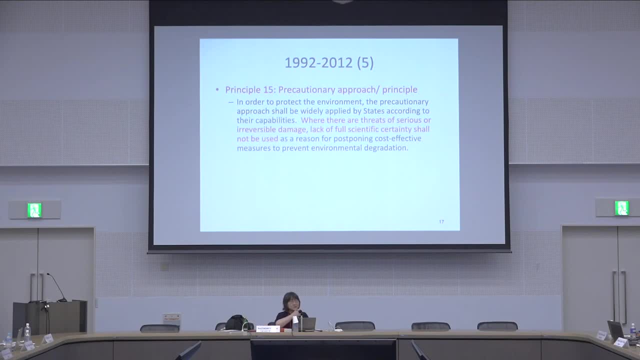 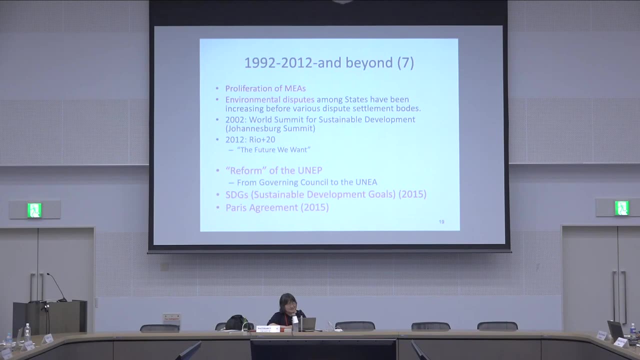 so it's a kind of example of application of precautionary approach or principle. so, uh, i, i now you know, the uh, you, you see that the uh list of material environment agreement which are now, they are rather the prolific, prolific, prolific, dated, and also the you know. 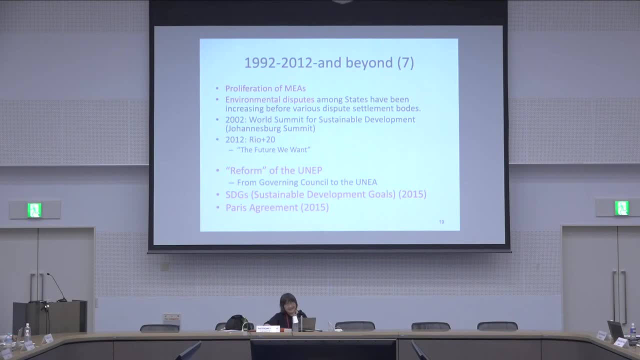 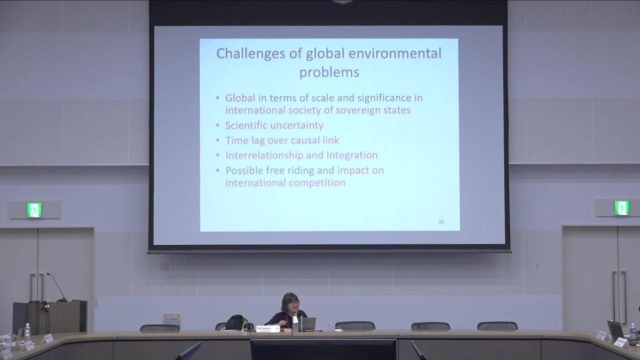 the important agreement made the sdgs as a long-term goal. i mean 2030, go political, go toward 2030 and the 2015. we see agreement of paris, agreement. i think we come back now later. so that is, uh, almost the very brief history of the international. 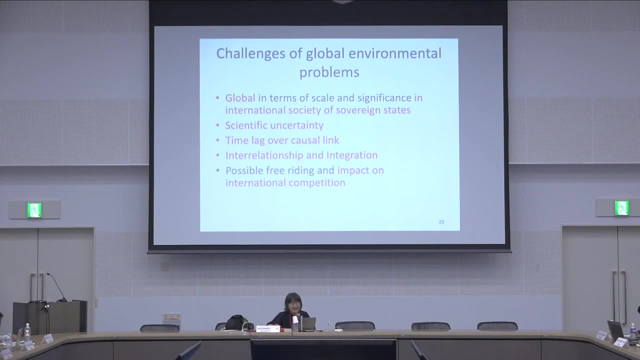 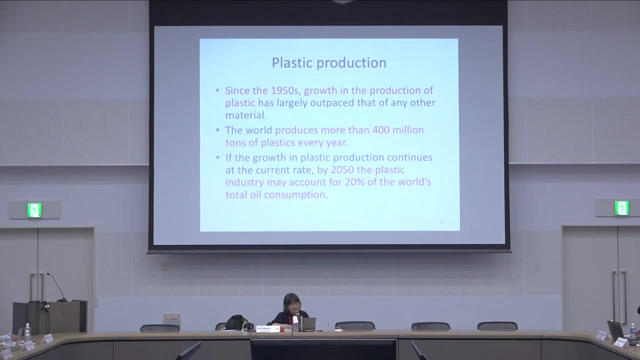 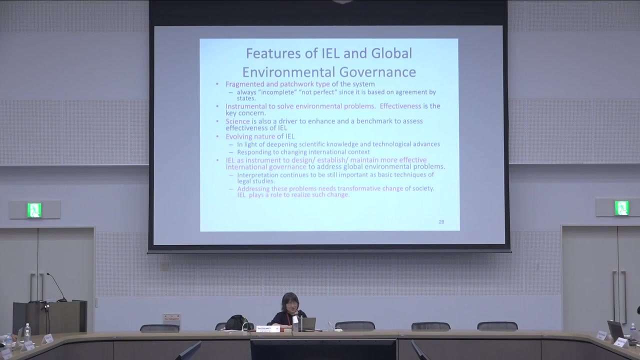 environmental law and the core obligation and the principle um this global. i could say that international environmental law has, uh, quite uh challenges and also features. i i go to the slide 28. one is that the, as you know, that not only in the environmental areas but also other areas as well, but often the country's 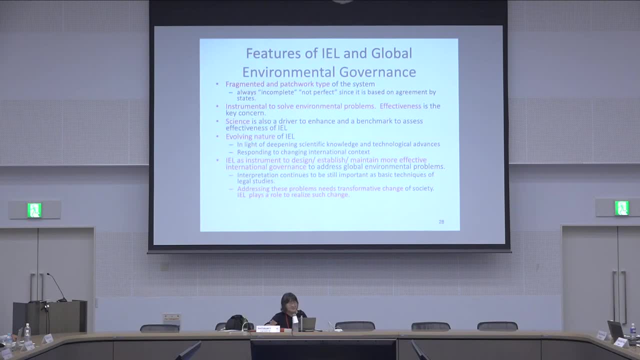 states agreement are piecemealed and fragmented depending on the topic that country agreed to negotiate. so the environmental- if you look at the list of machete environmental agreement, it is elaborated and agreed, agreed. you know the depending on each topic of the environmental issues, although they are very much linked. one example, i think, here: 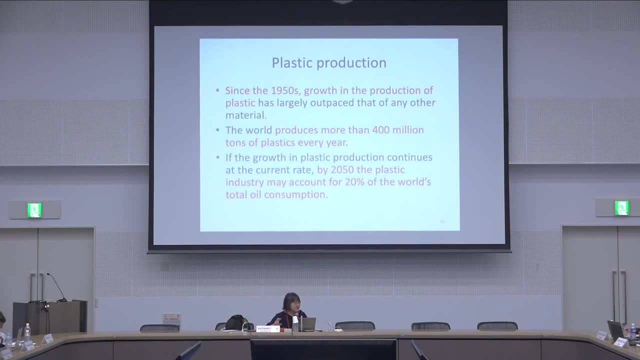 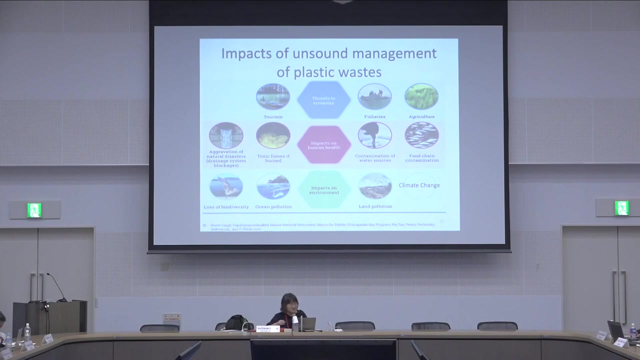 i just appeared. now we are go, we are doing the negotiation of the plastic convention treaty. but These plastic issues not only the environment issues, but also they have a lot of impact. Of course, if it's burned, it is burned, You know. usually it is made of. 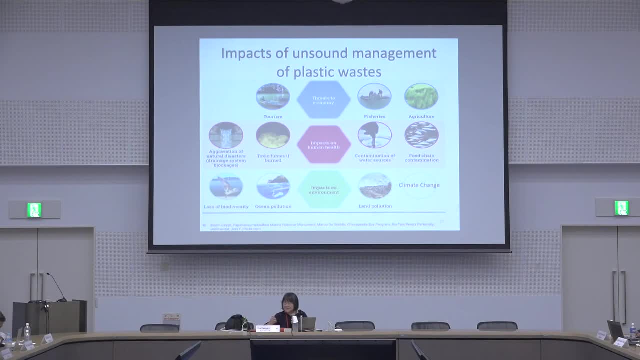 if it is made of the fossil fuel oil, you know it's emit the CO2, then it is linked with the climate change issues, Of course, the ocean pollution and the land pollution, and then you know, through this pollution, 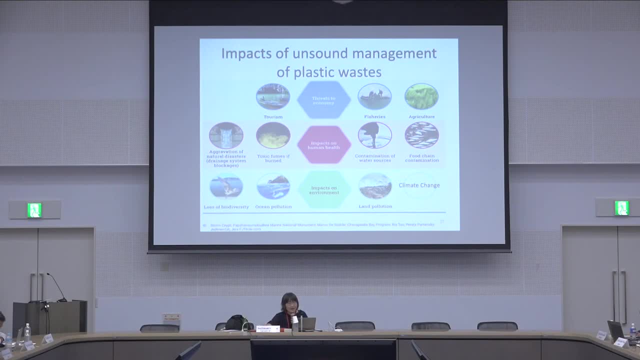 maybe we have an impact on biodiversity Through such a degradation of the environment. you know that might impact agriculture and the fisheries economic activity and the food security and others. So actually the issue are very much interlinked but, as I said, that international environmental treaty. 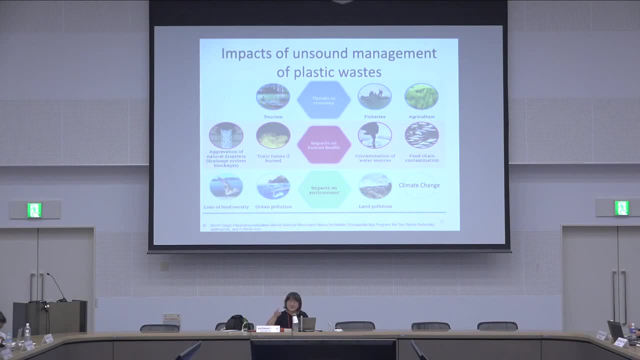 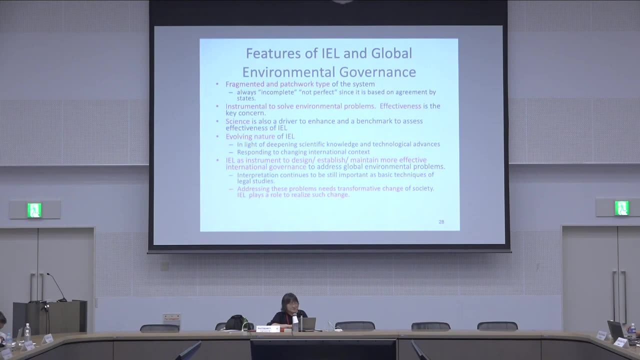 is usually elaborated on one specific topic that the country agreed to, So we can negotiate. So second feature of international environmental law is maybe different from the human rights law. Human rights law actually stipulates the absolute value to be protected under international law or between countries. 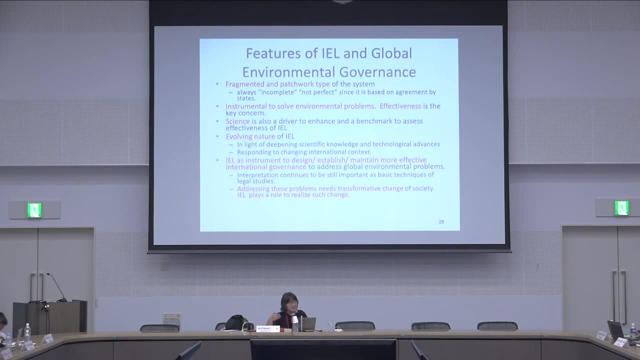 But international environmental law, multilateral environmental agreement treaty- it is rather provision of the multilateral environmental agreement is rather provide for how to approach to the in order to solving the specific environmental issues. I could say that it's a lot of the instrumental. 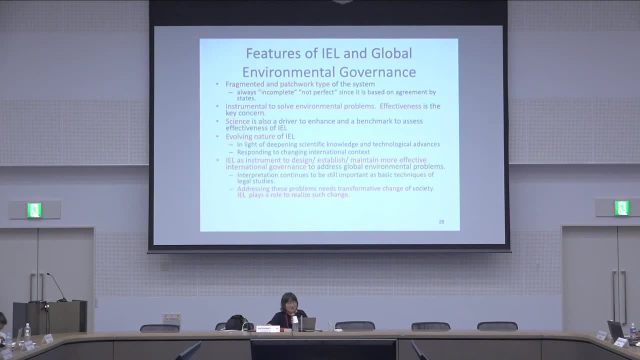 different from the human rights law. So what I could say is that the, as you know, you are the representative or official of the countries. you know that the any negotiation could not agreed if the one country strongly objected. So the that mean that the agreement among country. 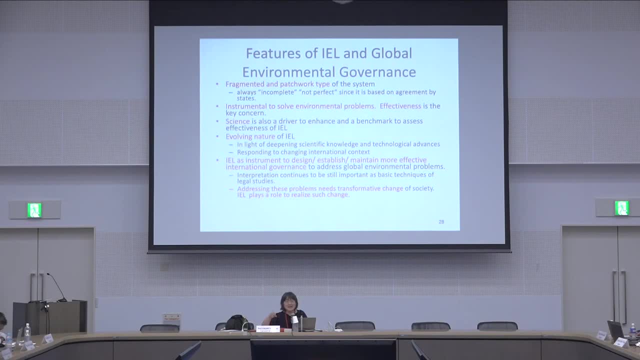 is kind of minimum level that all country agree. So, environmental issue: you know environmental agreement is to solve the specific environment problem but always insufficient to, you know, solve the problem Because country could not agree the you know ideal, the full agreement to tackle this problem. 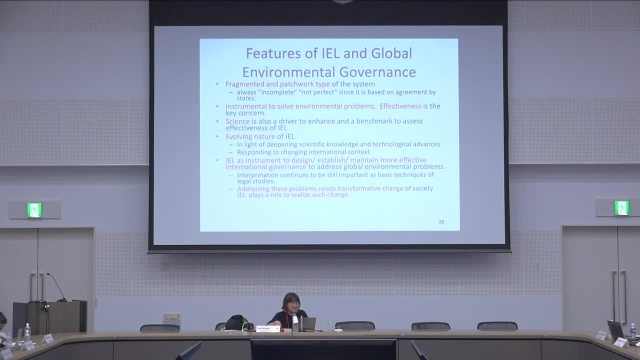 So, for one of the reason why, that is the reason why the international treaty on environment is always consistently above, Because the country's agreement, you know, upgrade up, you know the level that's actually the laser level of country's agreement. 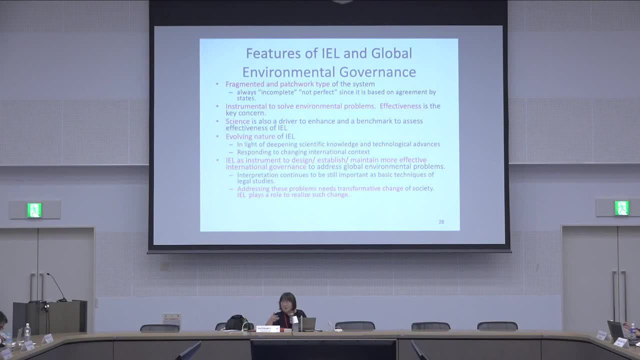 And so often the science developed over time, and technology as well. Then, as I said, even for the, from the start the level of agreement is very low, but over time we could get quite a sufficient level of the agreement, Maybe supported by science or technology. 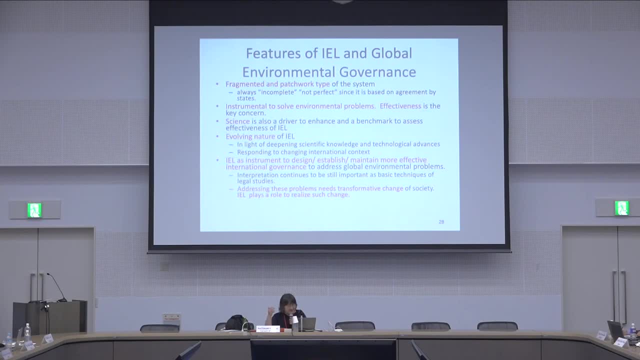 and the country agreed to you know the sufficient level of the action. So I could say that the international environmental law is always has evolving nature, especially that it's supported of every year or two years time conference of parties. So I think it's very important to nature. 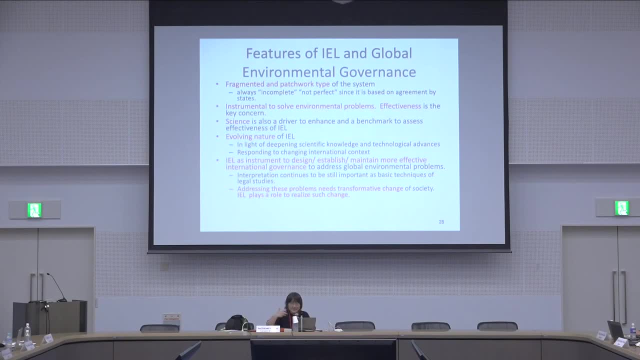 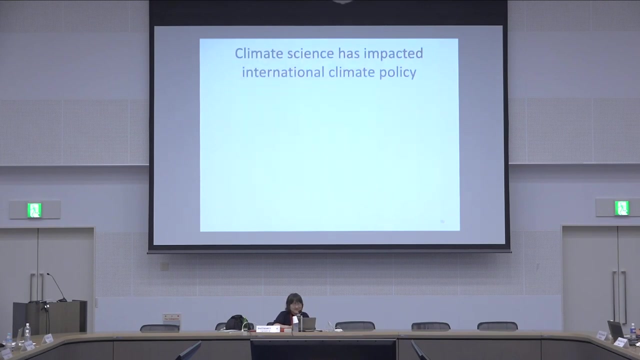 and that means that you could somehow elaborate a scheme to upgrade the level of agreement, That is, the wisdom of the country to negotiate, because once time, negotiation does not reach the sufficient level of agreement to tackle the environmental issues. So that's why I'd like to briefly 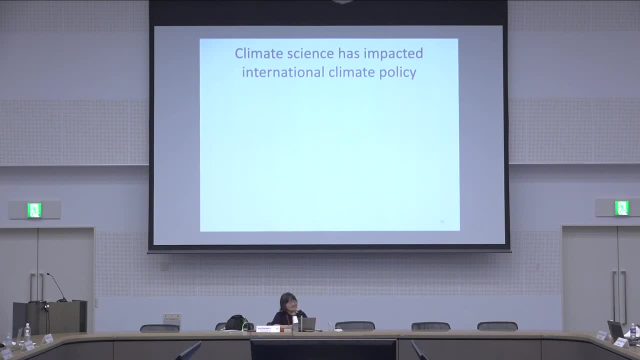 I think already, time is quite limited, but go to the climate change negotiation and the climate change law. First point, I'd like to say that I say that the international environmental law is evolving nature, often supported and driven by science. Climate negotiation is a typical one. 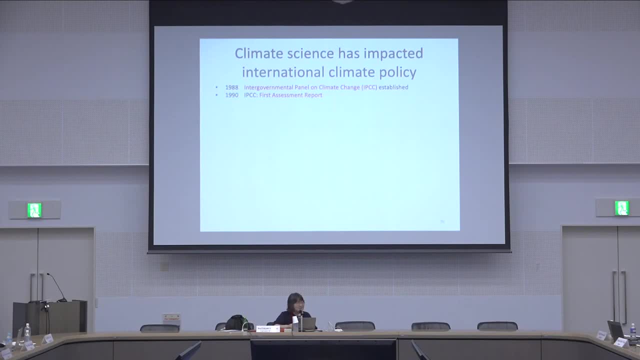 First, you might know that the climate science is somehow the. You know the reported by the international intergovernmental panel on climate change, established under the United Nations and UNEP and the World Meteorological Organization. It was established in 1988,. 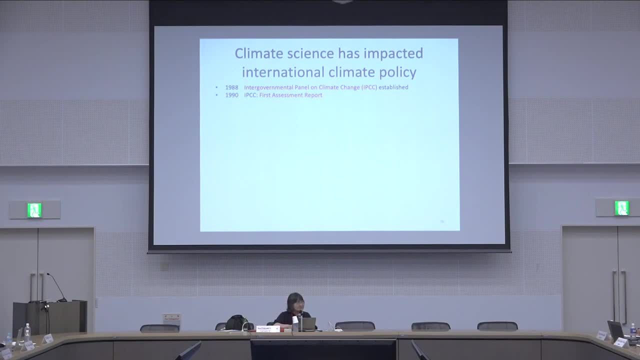 and the first report issued two years later, in 1990.. That's become a basis for the adoption of the United Nations Framework Convention on climate change, the first climate convention. So the second report come 1995, and that become a basis for the negotiation. 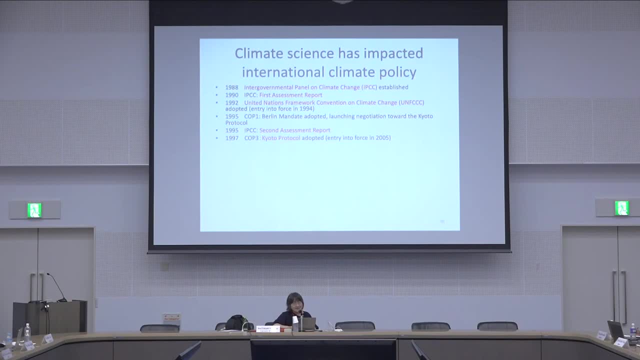 toward the Kyoto Protocol. That is the second international treaty on climate change And the third report come 2001,. that is, provide a scientific basis for the implementation negotiation of the implementation rule of the Kyoto Protocol. And the fourth report come at 2007,. 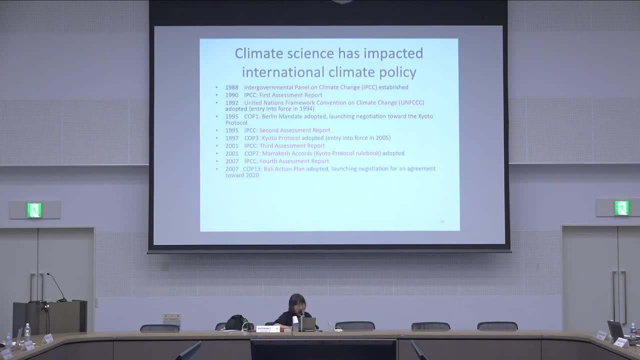 and that's trigger the negotiation, new phase of negotiation toward the agreement, toward the 2020.. And last, not the fifth report come. you know, the came at the 2014,. it's become a basis for Paris Agreement And then we just 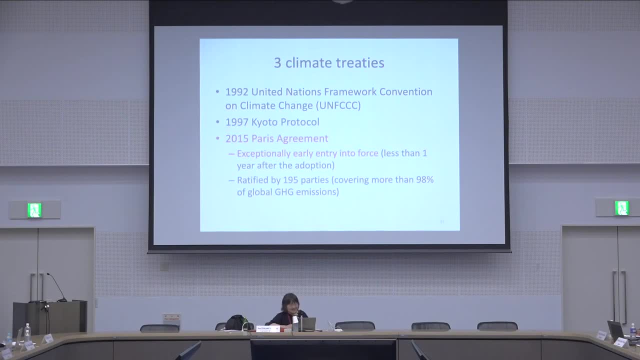 had six assessment report issued from 2021 and this year. So this is the three. already I mentioned the three you know treaties- I think you definitely know three- And Paris Agreement, already ratified by 195 parties, So covering more than 98% of global GHG emission. 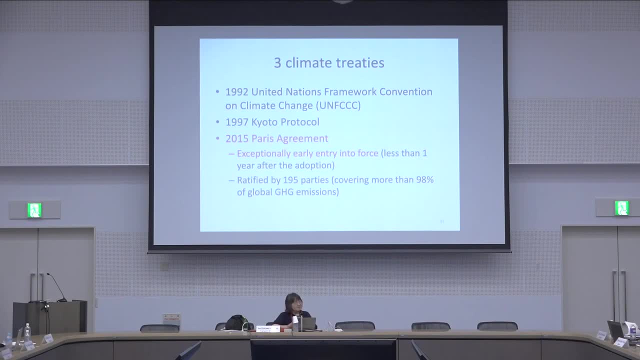 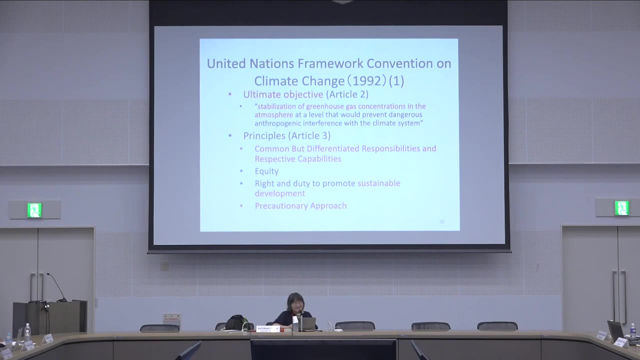 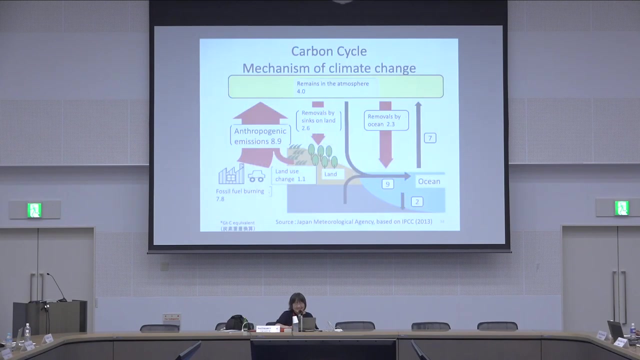 I think such kind of coverage level and never reached with the Kyoto Protocol. I'm sorry for that, But this first convention is only provide for the objective, long-term objective and the principle you are quite now familiar with, And that's rather the establish institution to say. 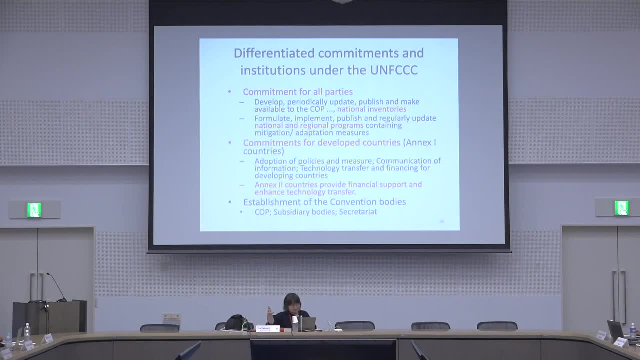 I say that's the laser level of agreement. so the every year the conference of party is held and to negotiate the agenda related to the climate change, And here the very basic commitment stipulated, commitment for all party, but only submit the national inventory of the emission. 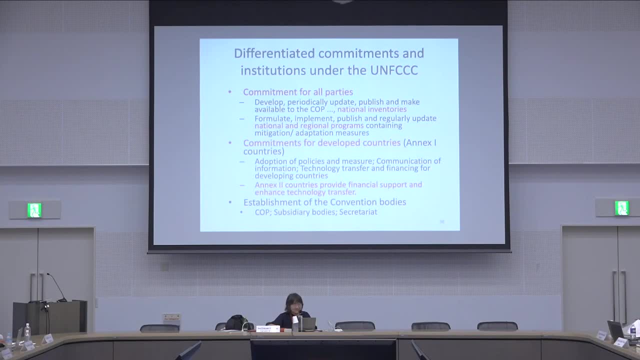 and the national plan containing the climate actions. And here you can see that some kind of differentiation of commitment between developed and developing country. under this first convention There are the commitment only for developed countries, some kind of, you know, more specific action to tackle climate change. 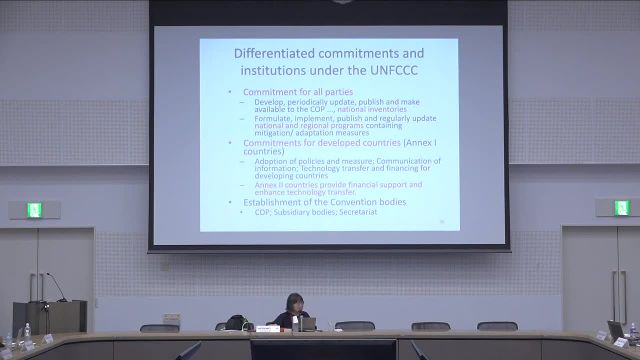 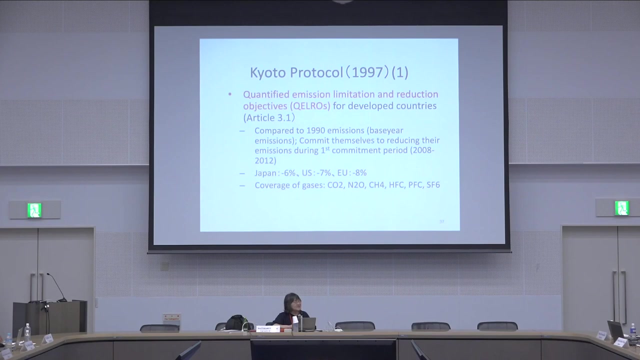 And also they provide the financial and the technological support to developing countries. It is only for the developed countries. They develop to countries. a commitment only for developed countries. Kyoto Protocol is also follow the similar differentiation scheme: always application as application of common. 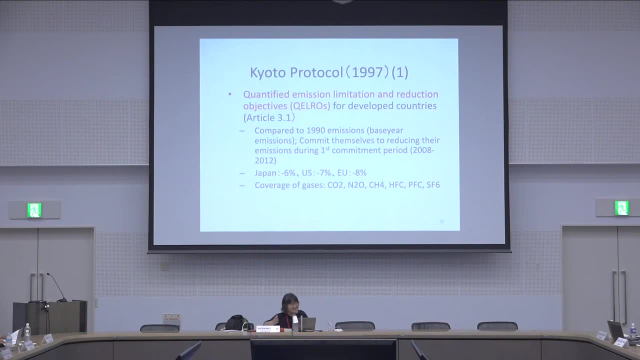 but differentiated responsibilities. As I say that it is a core, one of the core principle of international environmental law. But the Kyoto Protocol is a little bit different from the first treaty Because the Kyoto Protocol provide for the more specific numerical target to reduce emission for developed countries. 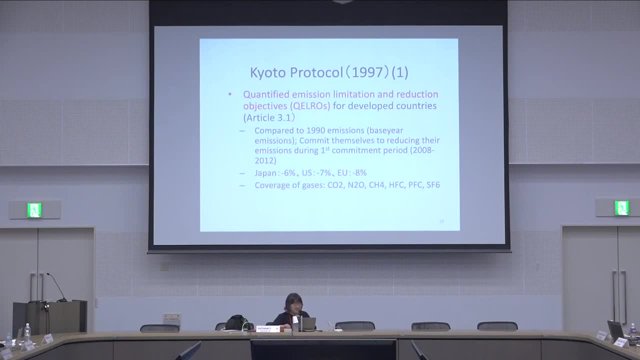 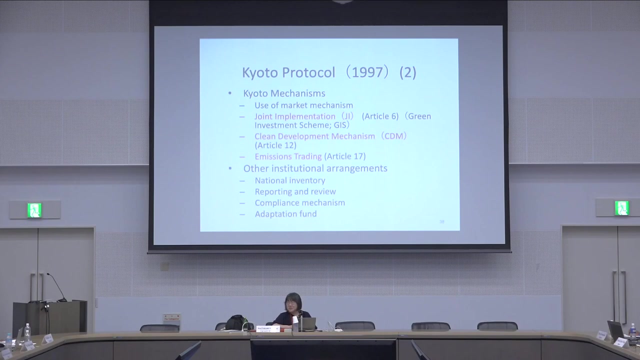 That I think you might be quite familiar. but there is no international commitment for developing country to reduce emissions. So differentiation in the followed as the first convention under the Kyoto Protocol. But the Kyoto Protocol somehow created an innovative scheme to reduce emissions, For instance the use of market mechanism. 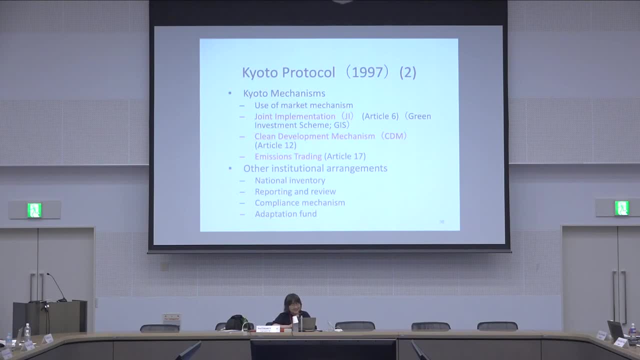 it's a carbon credit trading As established. maybe you might have a chance to know that clean developed mechanism, CDM especially. you know that quite a lot of project is emerged in developing countries And these market mechanism and the others institutional scheme is now carried over to Paris Agreement. 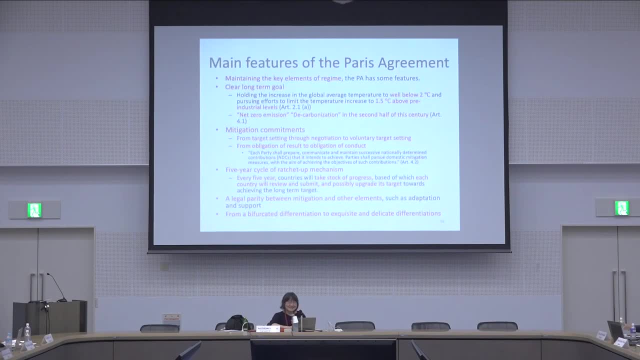 So then come to Paris Agreement. Feature of the Paris Agreement is one is the provide a more clear long-term goal. You know the, I pick up the. I hear the site, article 1.2.1A is that. 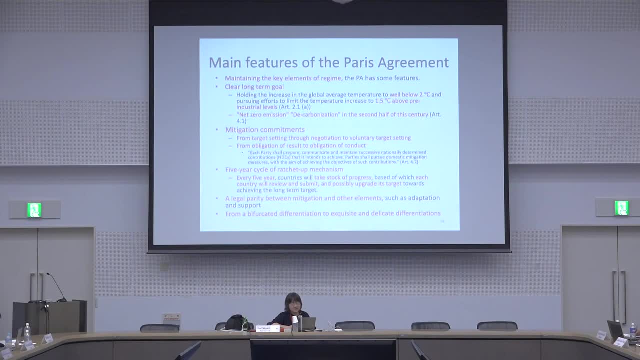 they hold in the increasing global temperature, average temperature to well below two degree and pursue an effort to limit the temperature increase to 1.5 degree above the industrial levels. That's correspond to need zero emission around 2050, in the middle of this century. 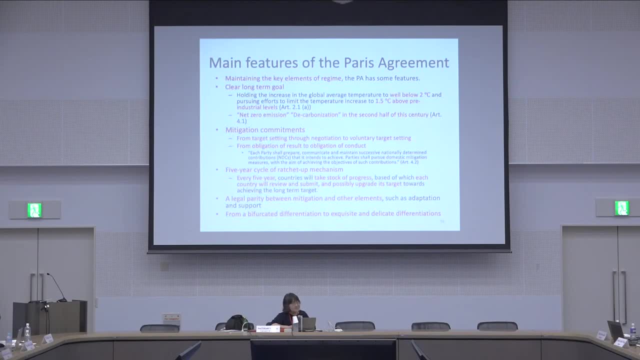 This is stipulated as mitigation goal or under the article 4.1 of the Paris Agreement. So often, then, the Paris Agreement provide a decarbonization goal. that's come from this, you know clause, and that's the article. 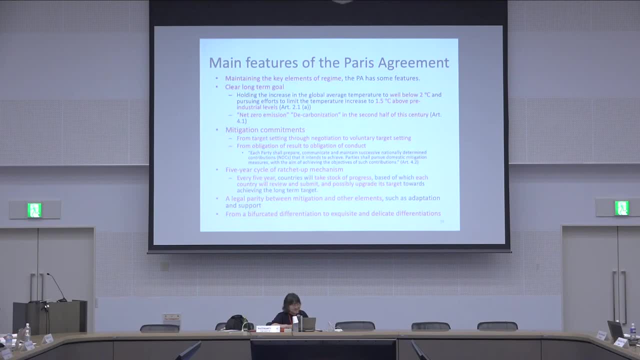 Another feature is the mitigation commitment. Maybe it's quite interesting because you can imagine Kyoto Protocol. you know the based on the usually in principle 1998 emission developed. two country have to reduce some percent. You know it's quite a, you know, common format. 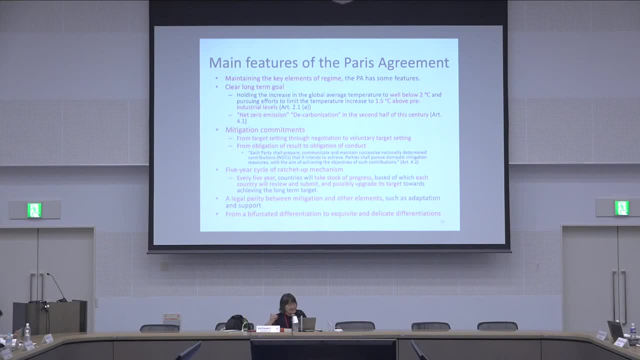 And then they once agreed this target should shall be achieved. If the country could not achieve it, you know they face some kind of consequence of non-compliance under the Kyoto Protocol. But here, under Paris Agreement, target level is set by each country. 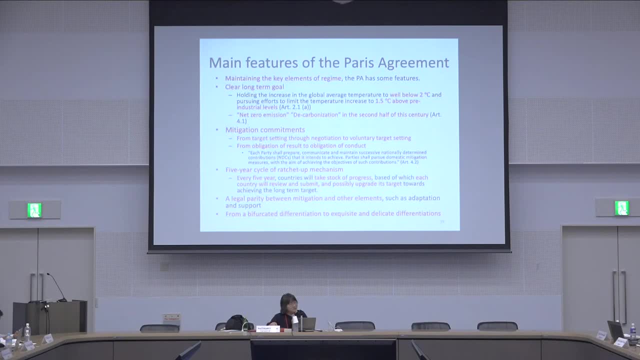 It's voluntarily set And also the you know level of target. as I said, it's voluntarily set, But if, after all effort, country could not achieve the level of the target, they cannot comply with the target there is if, after all, effort done. 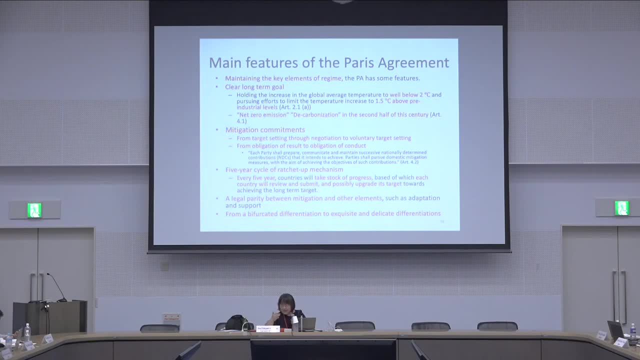 there was no penalty for such, you know, country non-compliant countries. So you can see this: the same- the Kyoto Protocol and Paris Agreement- is both a climate change agreement treaty, but approach relating to the commitment, especially the target of the national reduction. 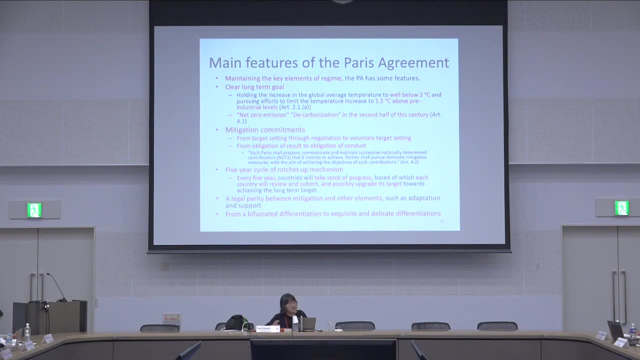 is quite different And also the compliance in case of non-compliance of the country. the approach of consequences against the non-compliance also very much different. And, the very last but not least, and the of course, the target level is set. 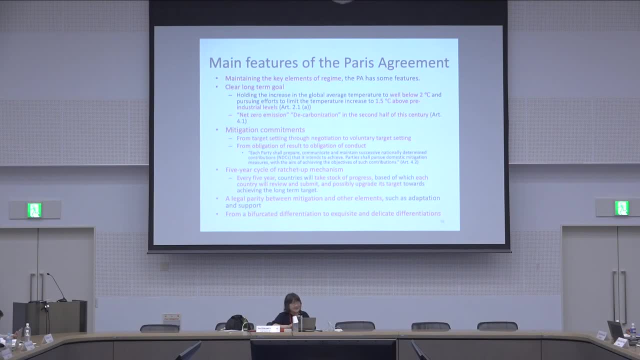 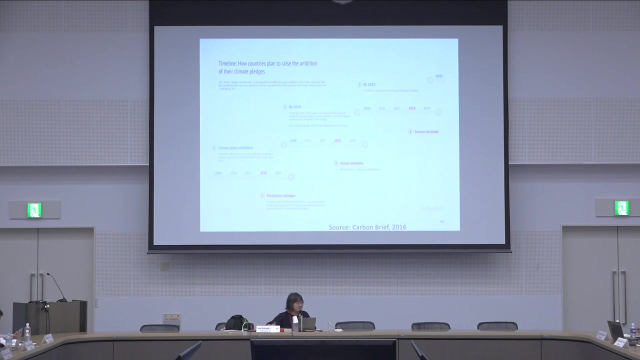 reduction level is set by each country, but every five years country have to submit again the new national reduction target. So that is the figure that you can see. Paris Agreement agrees 2015,. as I said, the five year. then the 2020, due to the COVID-19,, it carry over to 2021, but next time, in 2025,, all country, all party to the Paris Agreement, have to submit new national target by strengthening the emission reduction effort. compared to previous one. So together this is called the ratchet up mechanism, because every five years country submits the new target with more effort so that automatically the level of the emission reduction should increase over the world. So that is called the ratchet up mechanism. 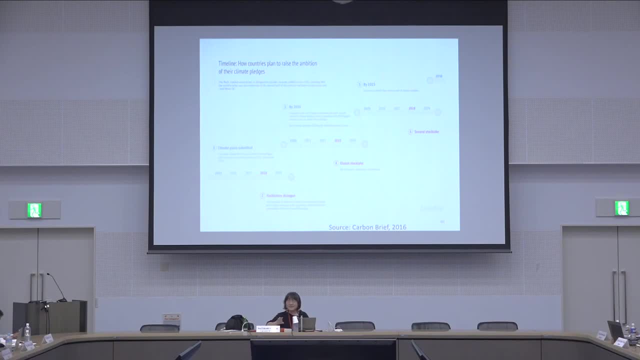 It's quite different of Kyoto Protocol, because Kyoto Protocol every five or seven years country have to renegotiate the target. So actually it takes much time and often I couldn't say often, but maybe could not reach agreement. 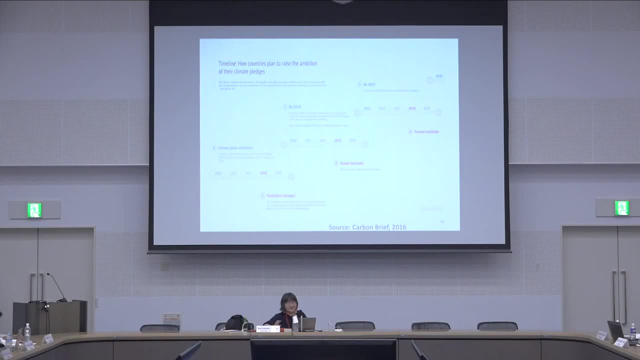 In that case there is no commitment under international law, under Kyoto Protocol. So this scheme avoid such kind of situation because of course the country have to submit everything they have to submit every five years. but still we can avoid. 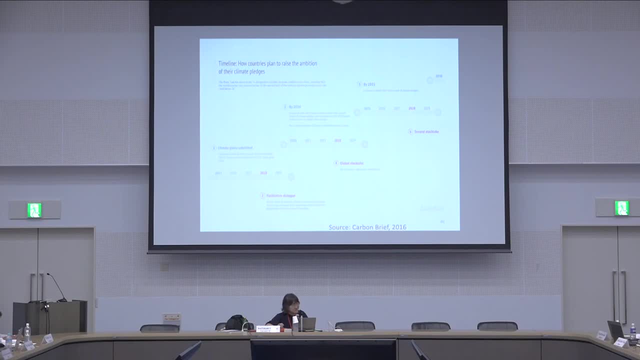 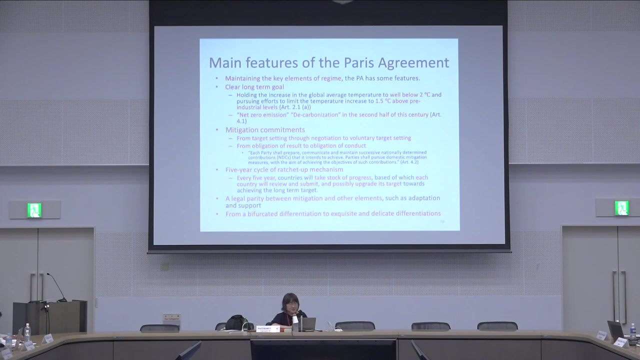 the no international commitment from each countries. Differentiation is also different from Kyoto Protocol. different from Kyoto Protocol because I say, under the Kyoto Protocol, together with the first convention, United Nations Framework Convention on Climate Change, it is some kind of bifurcated differentiation. 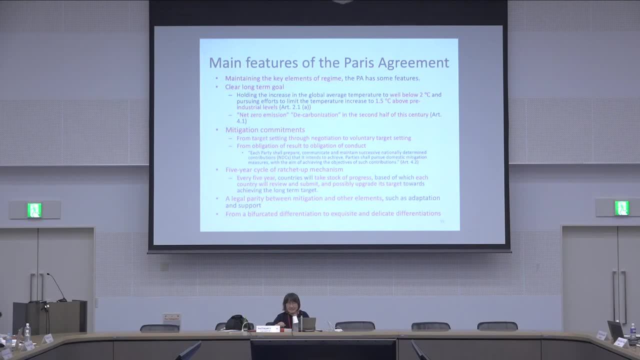 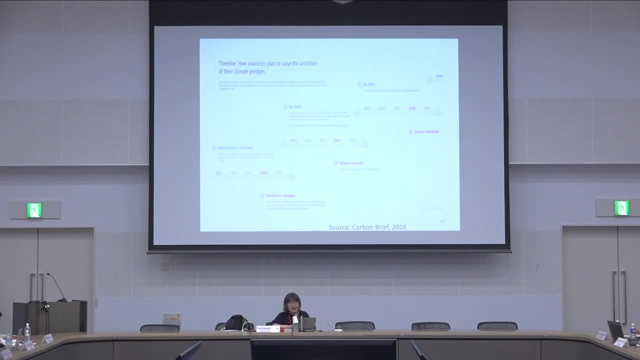 Differentiation between the developed country and developing countries. But now under the Paris Agreement differentiation of course made and allowed, but according to the national circumstance of each countries, And the differentiation then also should be converged over time. That is actually come from the proposal. 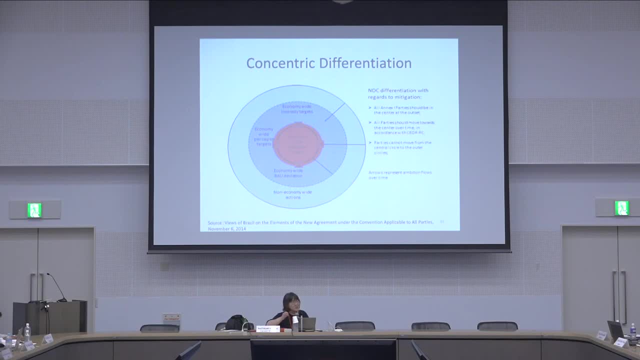 from Brazilian government because, of course, which status of differentiation that each country claim is, of course, the country decide. But once country decide, they try to diminish differentiation over time And finally all country have a similar national target over time. 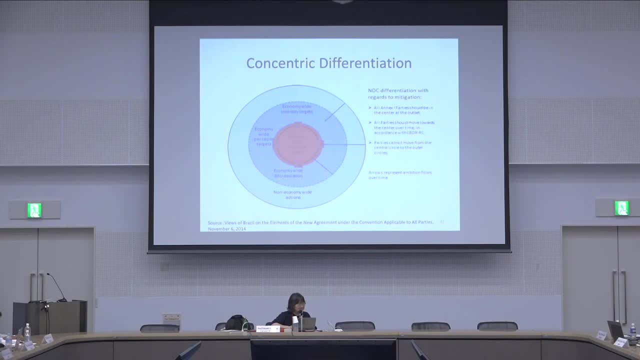 It is, you know, called the concentric differentiation, respect, somehow the you know, the difference of national circumstances, But over time we try to diminish and settle and dissimulate the differentiation over time. So this is a kind of lap up. 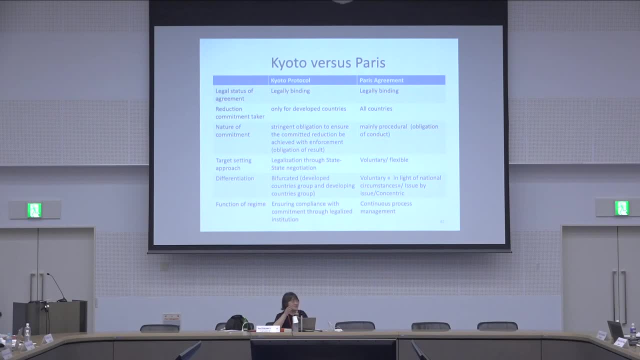 that what I told. I mean the even two convention, two treaty are relating to the climate change, but approach is quite different. We see what is more effective because international environmental law has objective to settle and address the environmental issues. So the how much effective is a key. 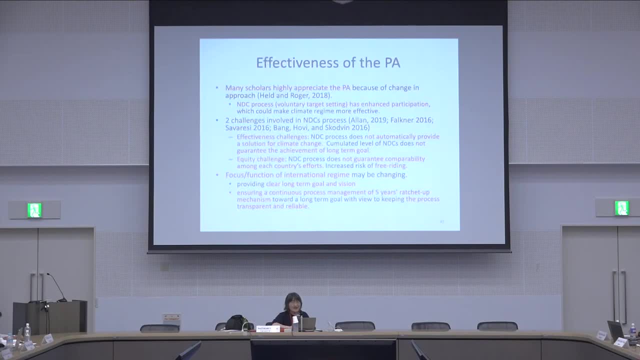 for assessment and evaluation. Researchers say that the it's a kind of success because it's covered broader countries with the national target, But still we do not see if it is sufficiently enough to be effective in addressing climate change, As you know that the climate change impact. 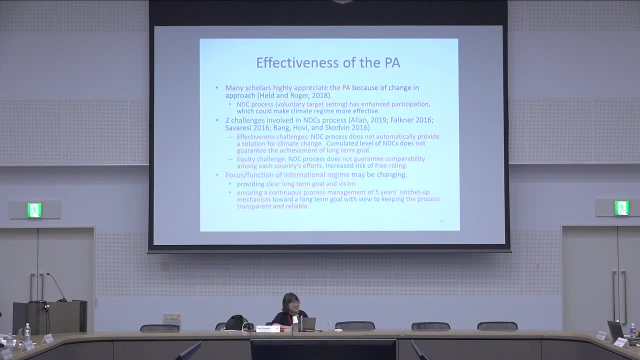 is now occurring and that we need accelerate the climate action. But is that the speed and scale is sufficient enough effective under this scheme? That is, I'm talking about Paris Agreement. And also equity challenge exist because the each country voluntarily set the target. 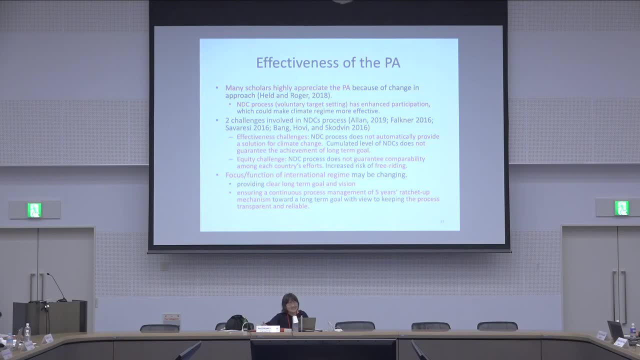 So automatically. it's not settle the equity problem. Maybe the similar country- country A, you know, submit, you know the some percent of reduction. but the similar country B with the similar situation, maybe not. you know less than. 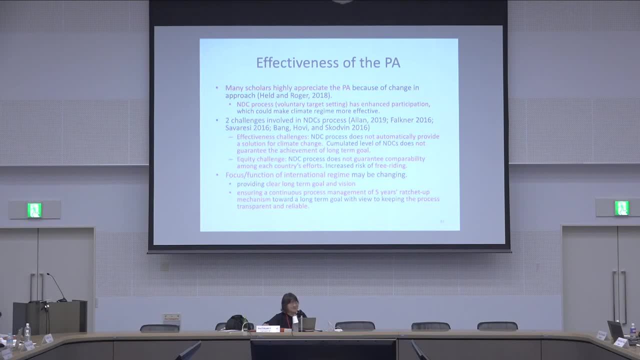 much less than emission reduction. You know the country with the similar circumstances, maybe not treated as like. So equity challenges exist, but still we see that some big. you know the move under the Paris Agreement, I think still we have. 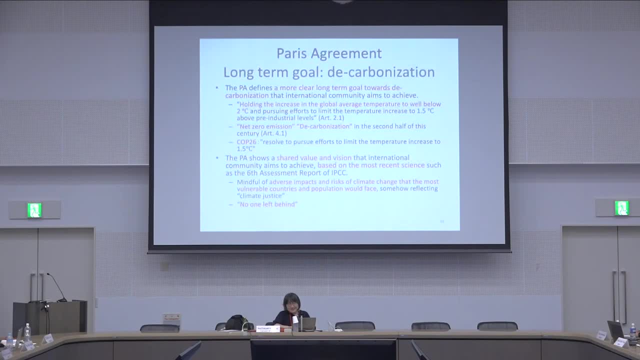 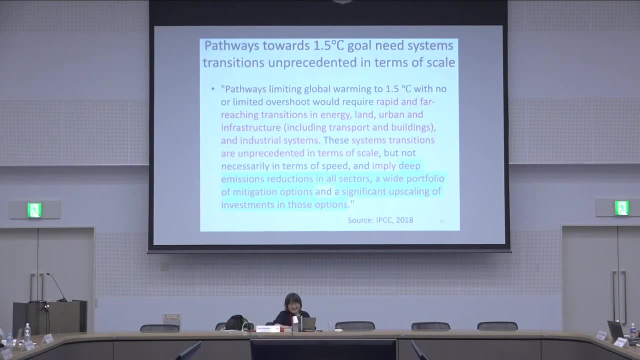 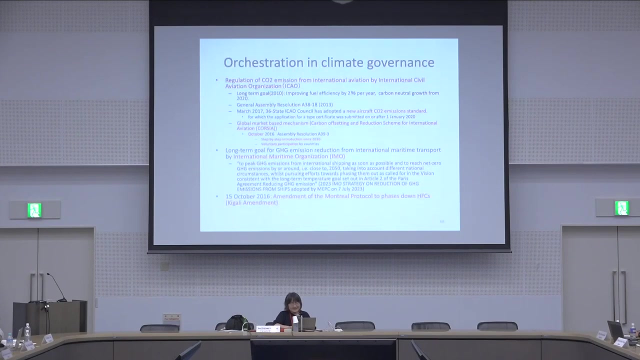 a little bit more time and I just focus on the some, because what I could say is the some new phenomena under the Paris Agreement. So one point is, I think this here: the slide, the orchestration in climate governance, climate law. 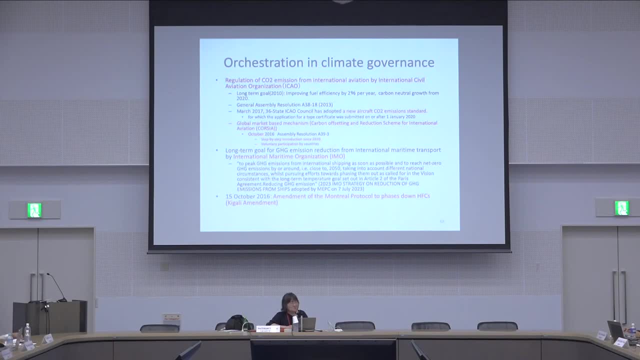 I told the Paris Agreement long-term goal That's direct to other international agreement such as the ICAO, International Civil Aviation Organization, which regulate the operation and environmental regulation on the international aviation international flight. So the now international emission reduction goal. from the international aviation is now the consistent with the Paris Agreement long-term goal And it zero emission by 2050.. The similar thing happened with the International Maritime Organization actually this July. This July, the International Maritime Organization upgraded the long-term goal. 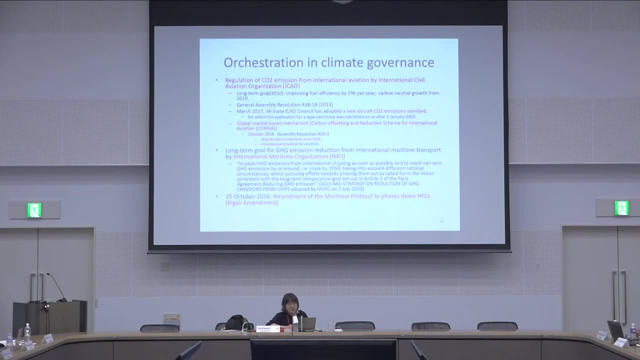 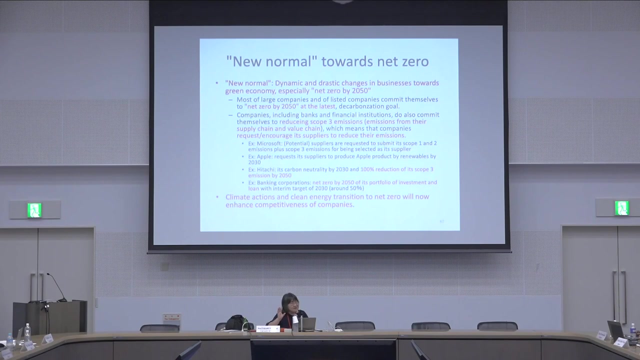 in a way consistent with the Paris long-term goal. The similar thing happened with the Montreal Protocol to regulate the some substances with the you know potent global warming. This is, that is the first you know phenomena that we see some kind of. 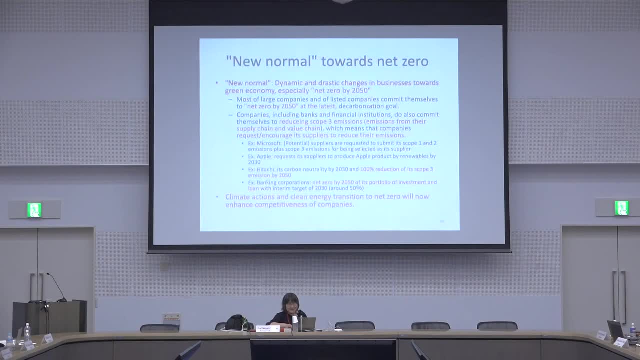 how can I say the? I could say some kind of extension of the climate goal to the other area of international environmental law. Second point that I like to say is that the, now the, the focus on the government, not the government. 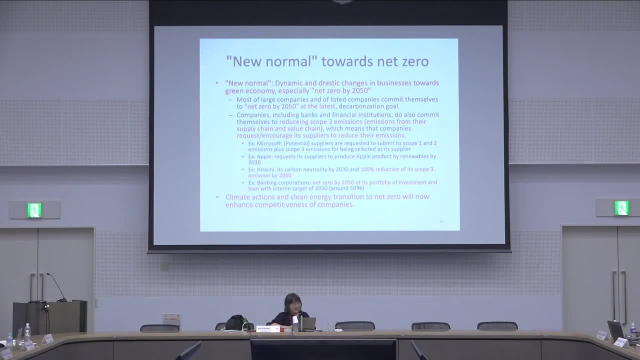 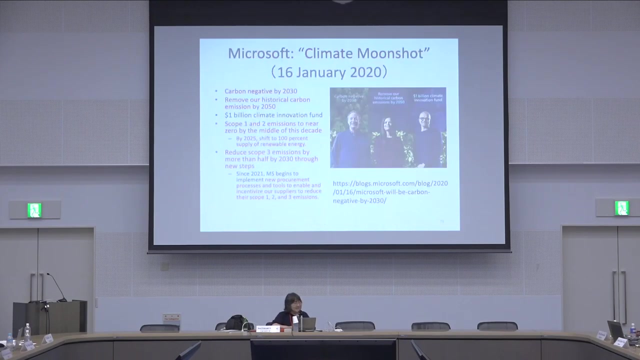 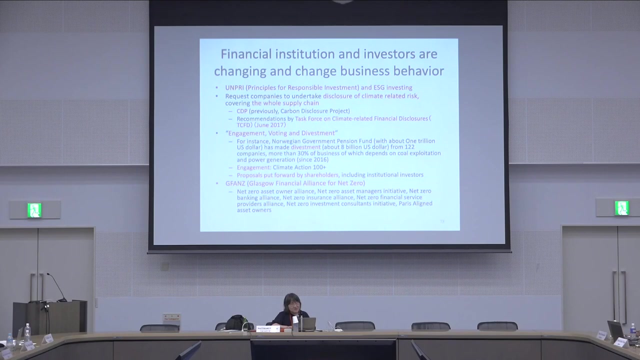 rather than the business and the companies. You might know that now the company is quite active in climate action. One of the reason is that they now, the financial institutions, very keen in the how the company react to this climate change issues. So the financial institution- 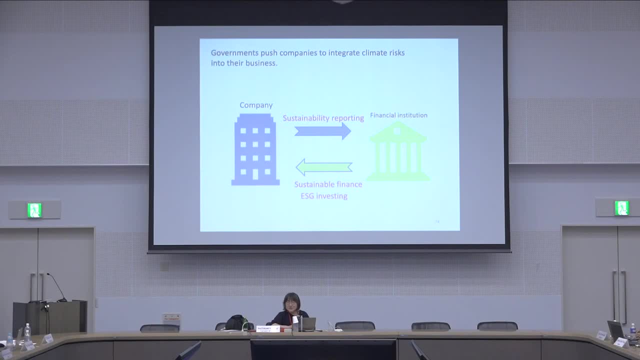 and ask the companies to disclose the climate related information and, together with the sustainability report, sustainability related information and then not only some kind of short term. you know the gain- business gain- but also the. you know how the company react to such issues. 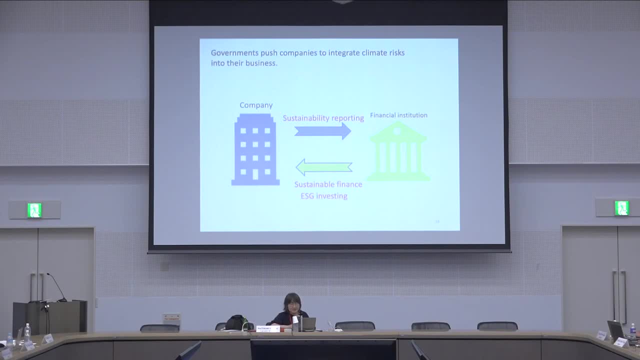 including starting with the climate change Financing financial institution, invest by the share of company, according to such information. So what I like to say is that now the many countries, especially the company, many countries, excuse me, many countries with quite a large scale. 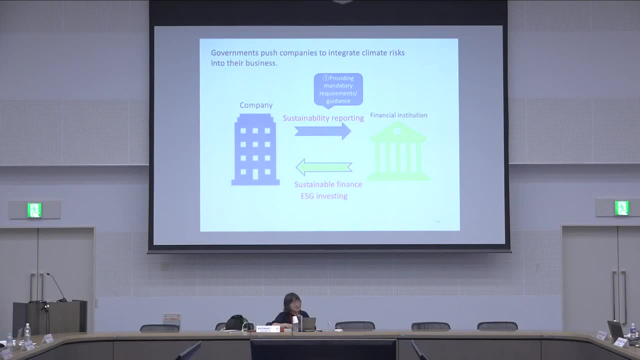 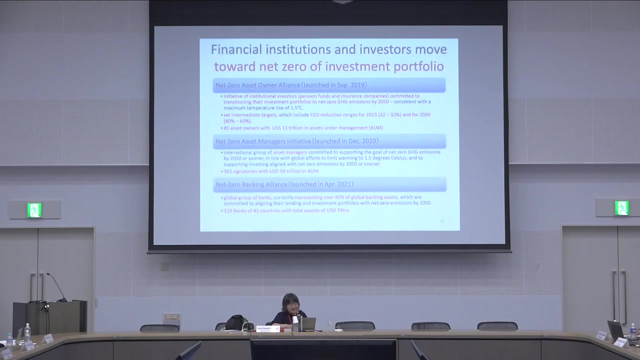 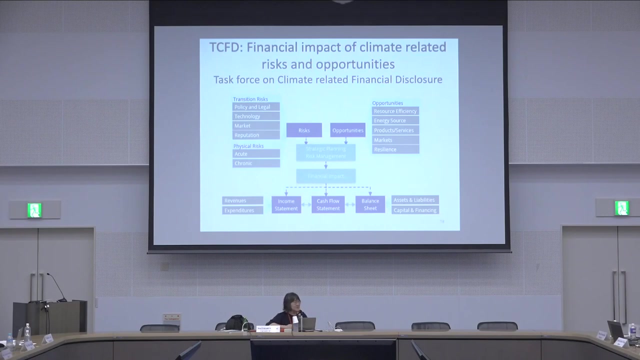 of capital market is now go. you know the act. now they regulate, they request, require the company to disclose such information under law. So I say here the how to say this figure is the some kind, yeah. 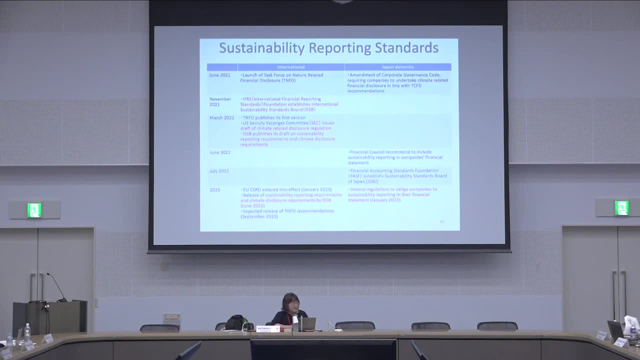 I'm sorry I could say this one Now: the international private entity- it is called international. you know the sustainability standard board, It is a private organization entity, You know. it create the sustainability reporting criterias which you know. 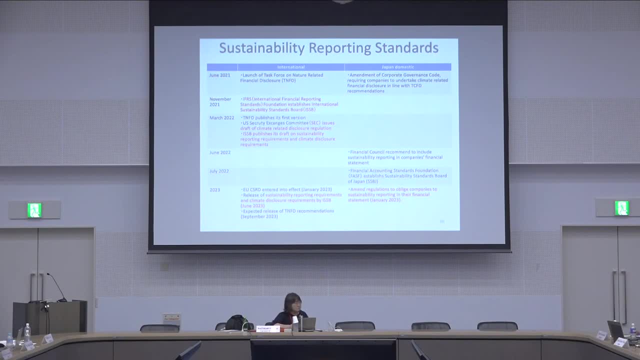 the. it is of course open for company to open to use or not, But this is, quite you know, the how to say now the many- I couldn't say many, but several country with the significant scale of the capital market. 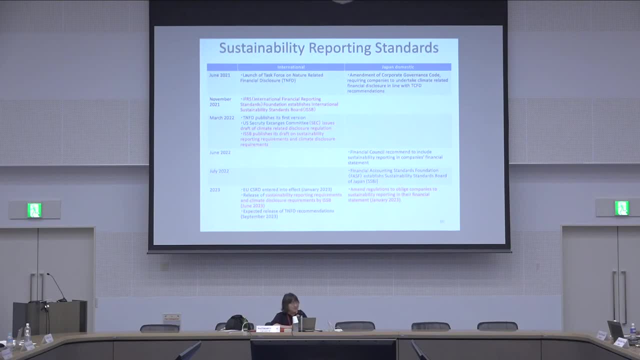 now introduce a mandatory requirement based on this standard. For instance, in case of Japan, you can see that the government amend the regulation to oblige company to report sustainability related information in their financial statement. So to report, of course they have to explain. 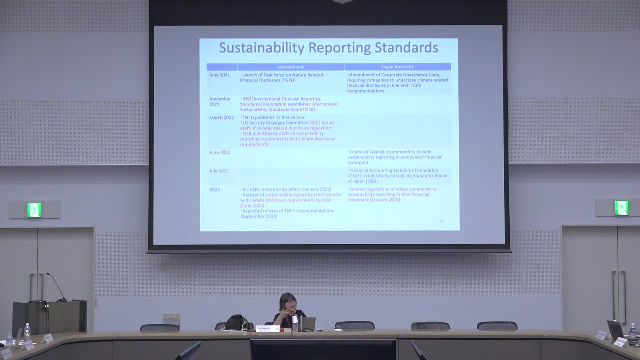 you know the how they consider the climate risk, how they the company reacts to climate change issues for from the long and medium and long-term perspective. So with that, the climate consideration are now integrated into the business management. So 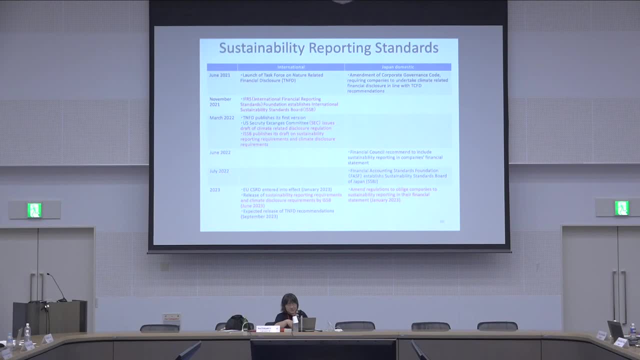 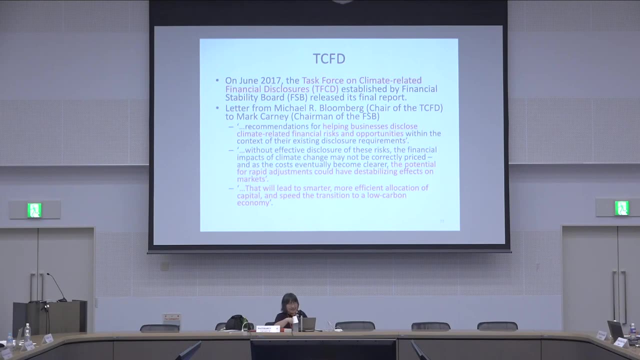 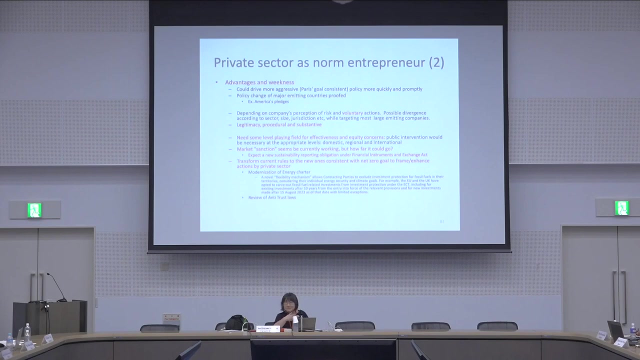 with that the financial institution try to assist, disclose these information and of course they assist the change of the business behavior toward more climate-friendly business or companies. So it is, I think, the very different from the Kyoto Protocol type. 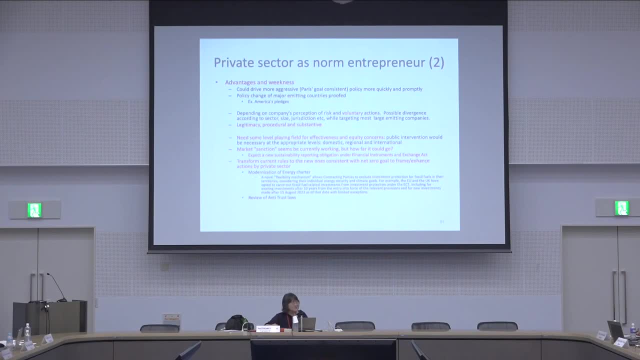 Kyoto Protocol period, because the private sector have a more, much, much larger role, and also in establishing international standard, for instance here, the sustainability reporting. it's not intergovernmental standard, It's a international standard, but elaborated by the private sectors. 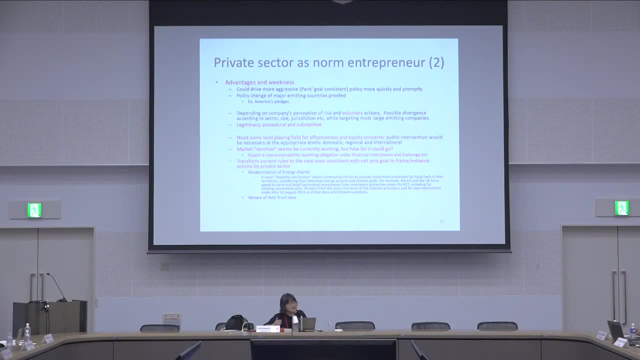 This international standard elaborated private entity, you know, rather go to the domestic legal scheme system and used by government and the company, you know, have to have a role and obligation to comply with under the each jurisdiction. So it's.